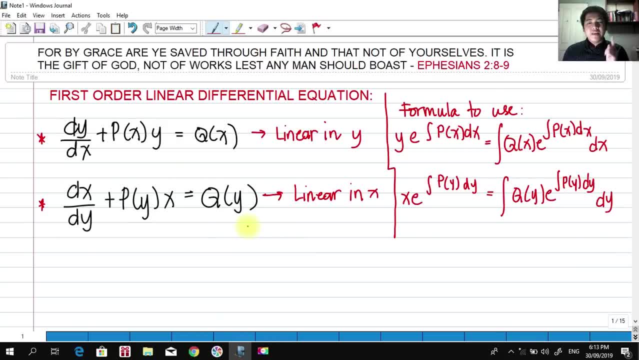 this formula. we say that the DE is a linear in x, as x is the dependent variable here. okay, So x and y are not the limited dependent and independent variable in solving differential equations. For example, in the application of DE we can see equations such as the change: 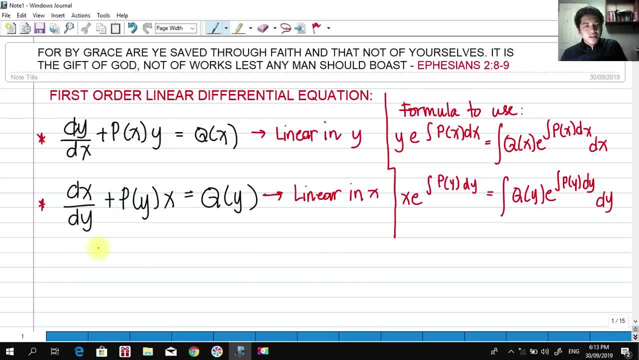 in current with respect to time, That is, change in the current with respect to time. So the change in the current is represented as i and the time is represented as t. So as you can see here, this is not the form of either of the two equations. So here is. 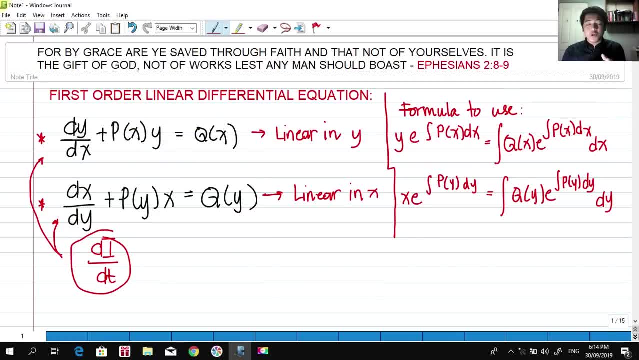 only the. I mean the form of which we can actually rewrite the DE. but that is not only limited in the dependent and independent variable, such as y and x. It can vary, For example, in the circuit we have di over dv, Where i here is the dependent and independent variable. it can vary, For example, in the 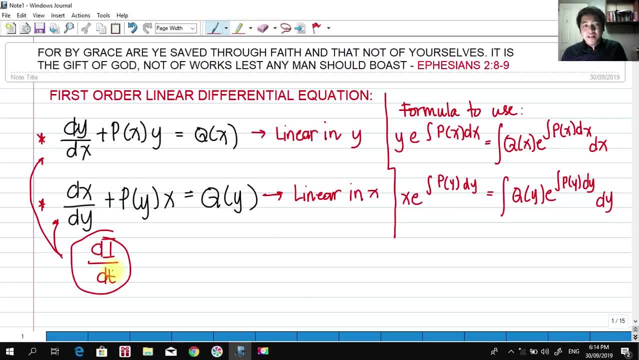 circuit we have di over dv, Where i here is the dependent and independent variable. it can vary, For example, in the circuit we have di over dv, Where i here is the dependent and independent variable. it can vary, For example, in the: 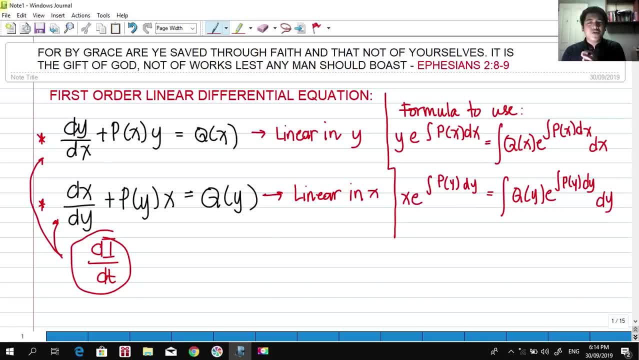 circuit. we have di over dv, So it can vary, But for some- not applications of linear differential equation of course- we simply use x and y. So if the DE is linear in y we have the formula to take note Wherein this side of the equation is: y multiplied by e raised to the integral of P of x is: 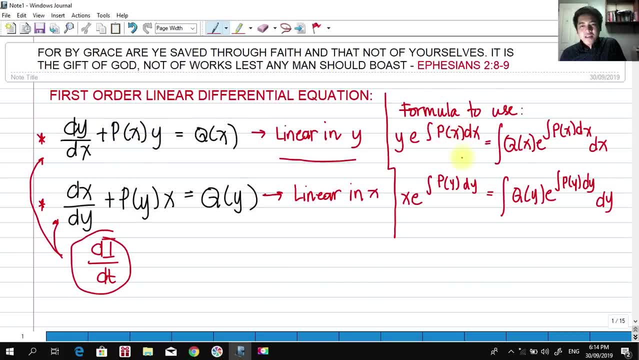 whatever p of x is here, okay, dx, and that is equivalent to the integral of q of x. here is the q of x multiplied by e, raised to the integral of p of x, dx, and evaluated in dx. okay, the integral is evaluated in dx. so what is this? e raised to integral p of x, dx. that is the integrating factor. 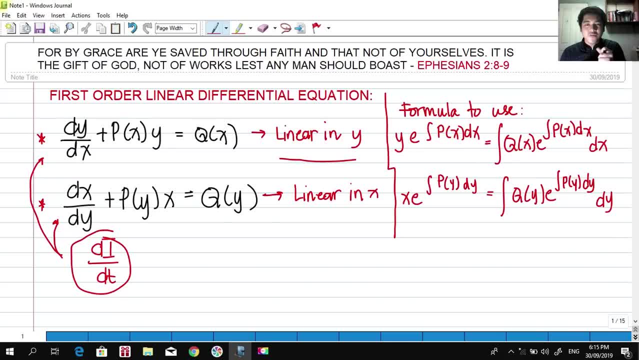 okay, but, but in our discussion for today, we're going to simply use the this formula, this following formula. we have a new monix here during my review time, so i don't know if that would be helpful for you- it we, we actually memorize this formula as: yes, pdx, Klast, pdx. okay so, but 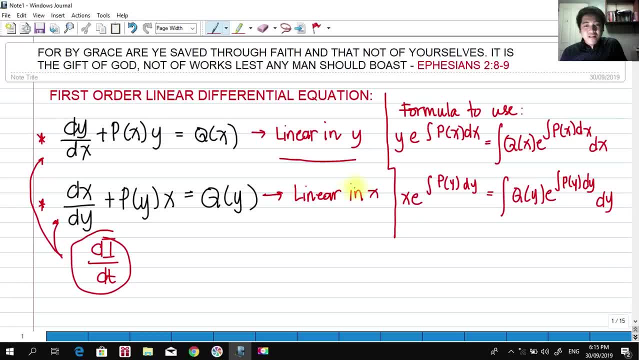 we can memorize this right. so if that is a linear in x, if the differential equation is linear in f, like this, we can memorize this okay. so we can memorize this okay. so if you linear in x, meaning we can express the d in terms of this form, then, as we can notice, 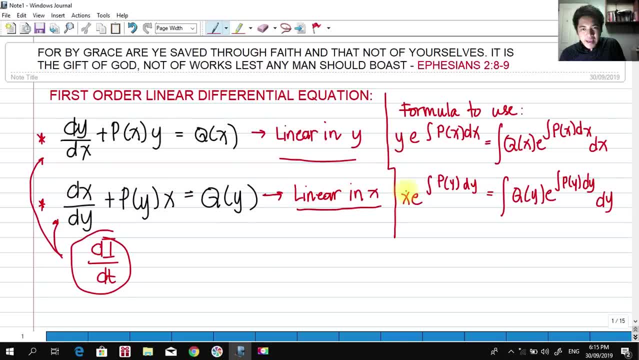 this y is simply replaced by x. so and this p of x simply replaced by y, and of course, our dx is replaced by dy. so same formula. okay, so we have x times e raised to the integral of py dy is equal to now to the integral of q of y, which is this multiplied by e raised to the integral of py dy. 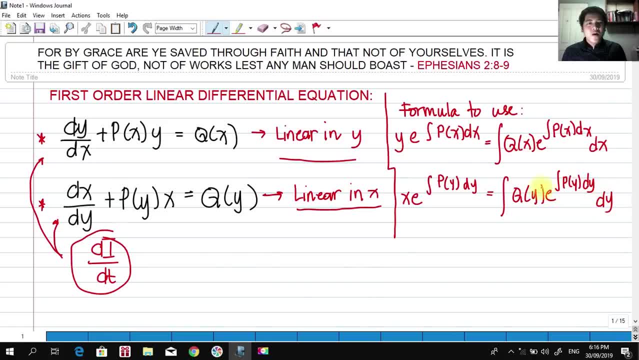 evaluated the integral in dy right. so in solving the linear ds it is important to actually memorize this form, or at least familiarize ourselves on how we are going to reduce the d in this form. because you must memorize this? because definitely, in order to you to solve d e linear d, you have to put the d in this form. if you are able to put the d in this, 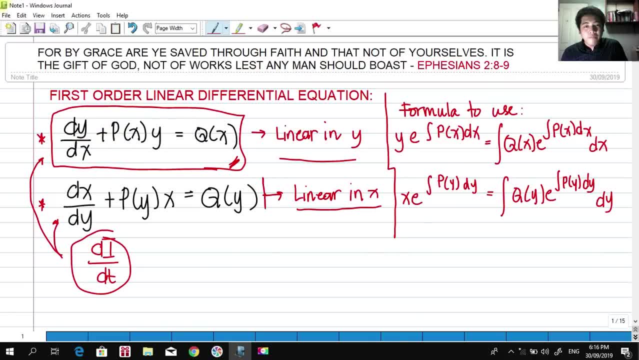 form, then that is said to be a linear d, or in this form in our second equation. and again, our dependent and independent variable is not only limited to x and y. so in applications of being you have the current over time here, so it varies. okay. so let's try this whole. so, for example, this example, so we 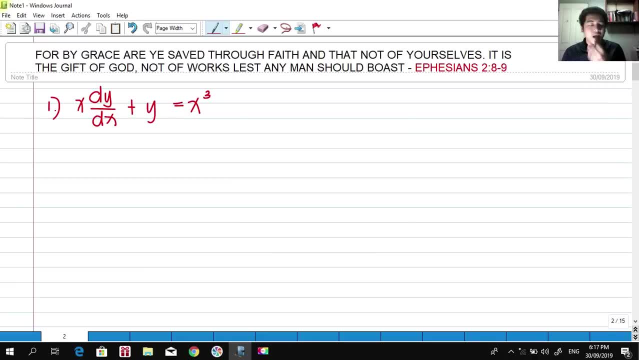 have x, d multiplied by d, y over d, x plus y is equals to x- q. so our goal here is to make this d look like in our- okay, look like in our linear in what? linear in y, right? so why did i say that is a linear in y? because definitely, if you're going to look at the dependent variable of this, 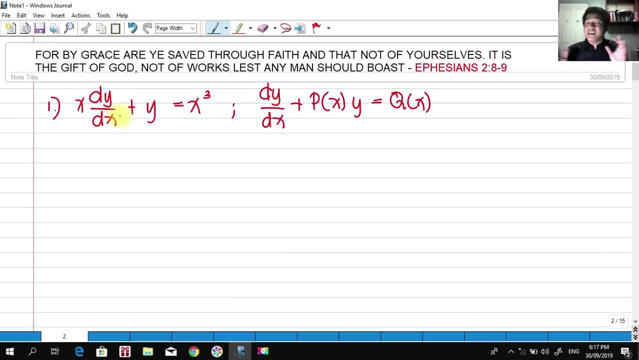 d that is in of Y. so I can say that that is a linear in Y and here is our formula or our form in linear in Y. okay, so I would make this DE look like this: so if I'm going to divide both sides or multiply both sides or divide both sides by 1 over X, so what? 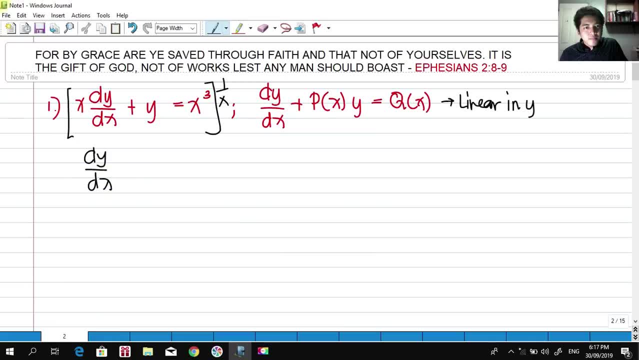 will happen. this should be DY over DX plus 1 over X multiplied by Y is equals to X squared. as you can see here, we have written this DE already in the form of this linear in Y differential equation, why we have DY over DX. that's a check we 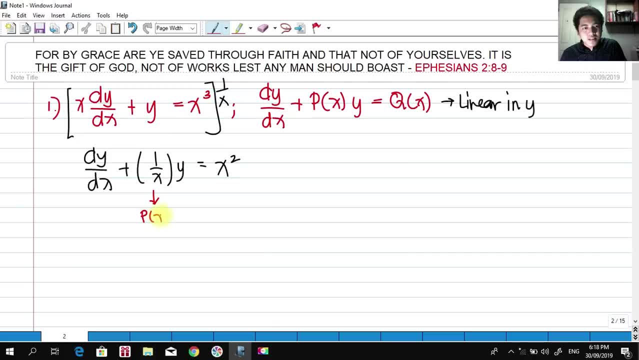 have P of X. this is now our P of X, okay, multiplied by Y. and this is now our Q of X. okay, and again a while ago, we have formula that if the differential equation is linear in Y, we can solve the DE by, okay, Y times E. raised to the integral of P of X, DX is now equal to. 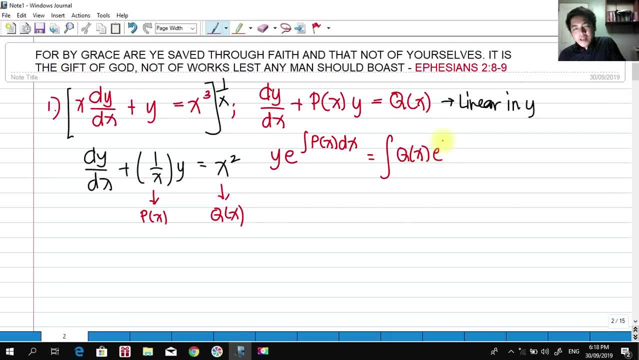 the integral of Q of X times E, raised to P of X, DX and DX here. so if we're going now to solve the solution for this DE, okay, we simply copy Y, because that's the formula. simply copy the E integral of P of X, DX. our P of X here is 1 over X, DX and that is equal now to the integral of Q of X. 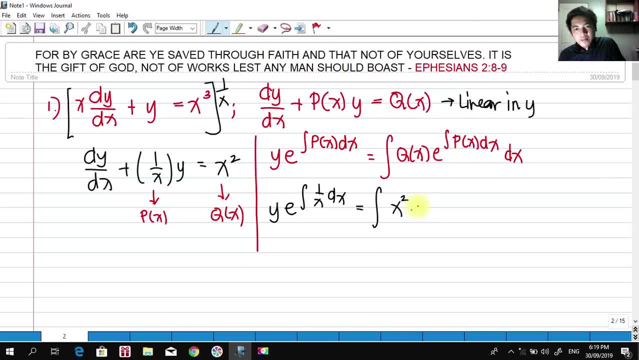 which is the x squared multiplied by E raised to the integral of P of X. again 1 over X, DX here and then. ok, then lastly, we have DX here, so we're going to evaluate this. Y E raised to this is simply integral of DX over X is equal. now to the integral of X squared, E raised to still the same, DX over X, DX here and then. now we're going to need to divide the drugs again. Y, hein, the numbers here are equal now. Q of X and discrimination. what will happen now? so you can see, we have Y dashed here and then, Mira, we can see all these. 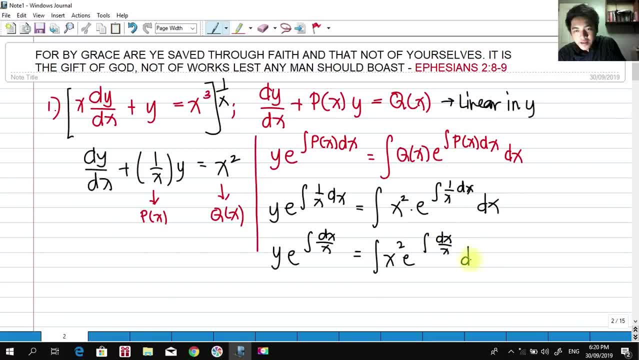 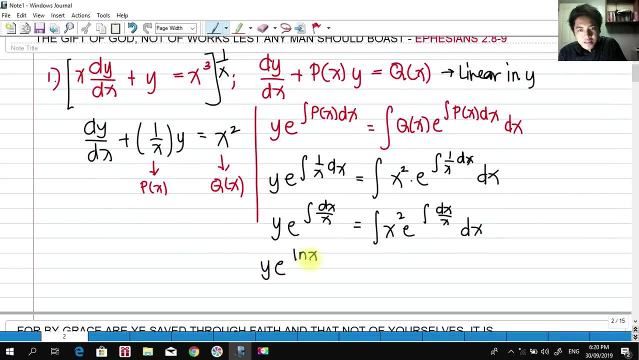 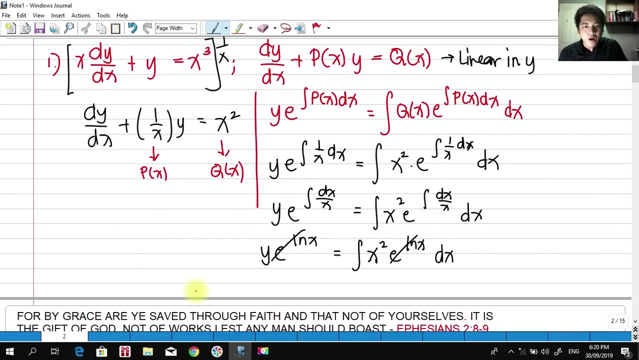 still the same dx over x dx here. so if we're going to evaluate this, this is y integral of dx over x is ln of x is now equal to integral of x squared e raised to ln of x dx. and, as we can see here, e raised to ln will cancel okay, and we are left with what we are left with: y multiplied by x. 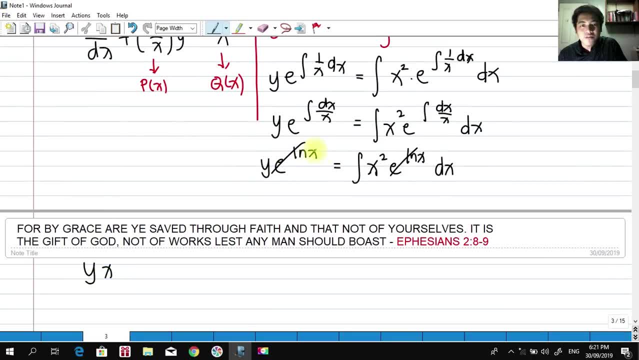 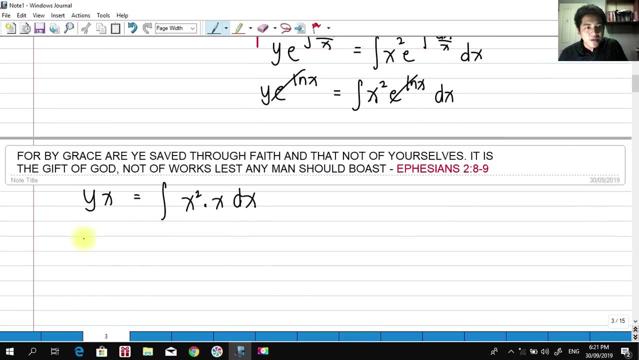 because, again, if we cancel this, the only term that would be remaining is the inside function of ln, which is the x. okay, and equal now to the integral of x squared multiplied by x, dx. so our solution would be: x to y, okay, integral of x cubed dx. so we have x, y, x raised to 4 over 4, plus a c. 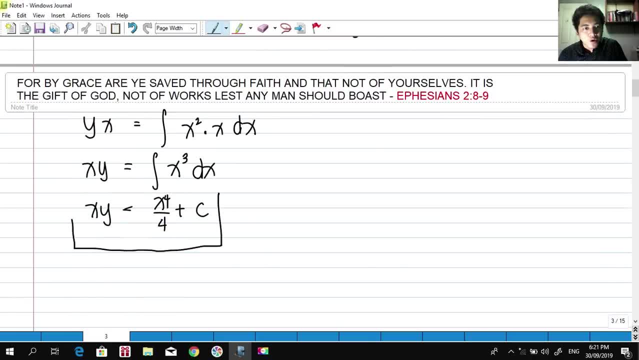 now, this is the solution to our linear differential equation. the solution or the final answer may vary, but as long as you are done integrating, as long as you are done, uh, done with the integration, this could be considered as the solution. but oftentimes, if you are having a multiple choice, 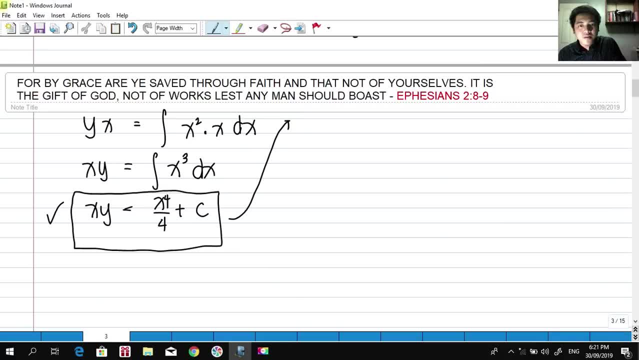 question whatsoever. okay, your professor require you. sometimes it is expressed in terms of y. so if you have that x raised to 4 over x squared dx over x squared dx, so this is the solution to our solution to our linear differential equation. this is the solution to our linear differential equation. 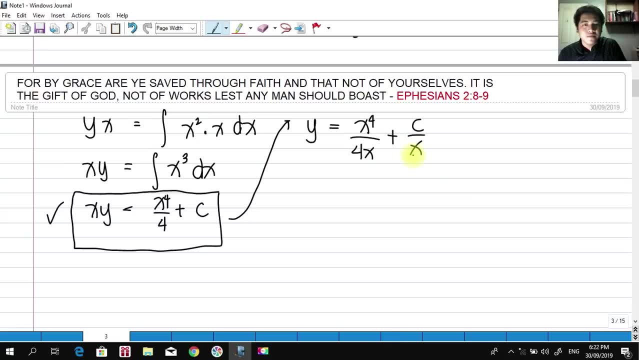 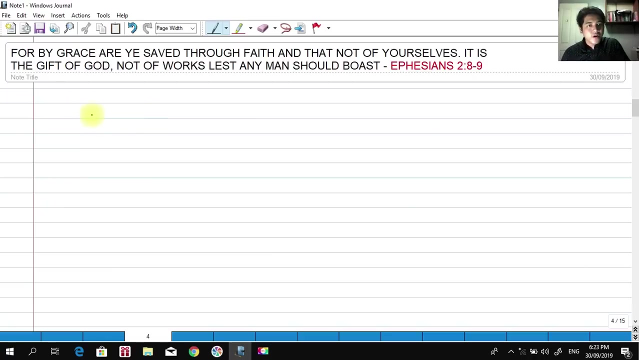 okay, so we have y is equal to x cubed. this should cancel, okay, over 4 plus c of x. so this should be can still be our answer, okay, so let's try again. another problem. so for our problem number two, we have dy over dx plus y is equal to e raised to 2x. okay, so this is an easy problem, right, because the the given d is. 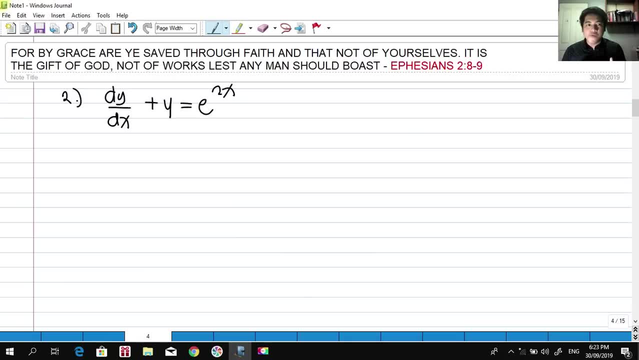 already in the format or in the form of dy over dx. plus p of x multiplied by y is equal to q of x. okay, so why did that happen, sir? we have dy over dx here. okay, of course that is a linear py in y, i presume right. so plus y, where is the p of x? the p of x here can be equal to one, okay, and it. 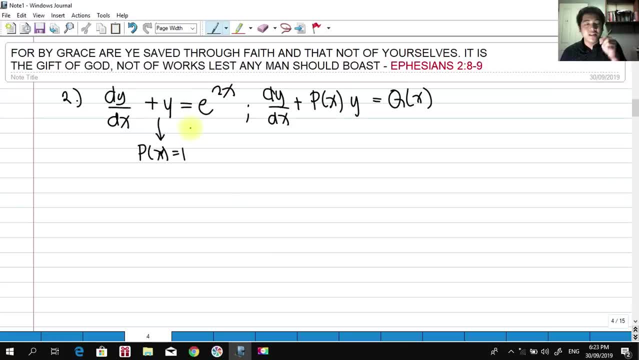 is equal actually to one, because one times one is one times y is still equal to one. so our q of x here is still e raised to equal to. oops, let me just rewrite: q of x is equal to a raise of two x. q of x is equal to, equal to a raise of two x, and this will solve this centimeters. so first, all we 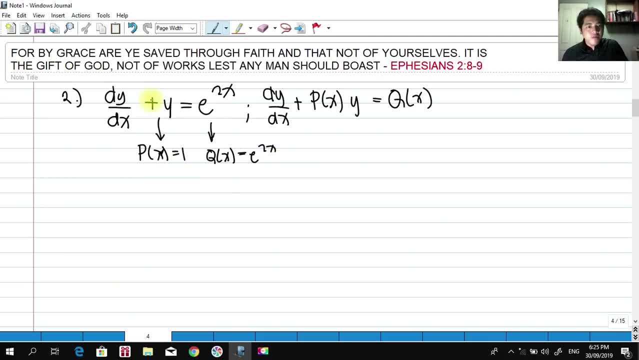 So we should use again the formula we have used a while ago, That is, y times e raised to p of x to dx is equal to integral of q of x. e raised to the integral of p of x to dx, then dx. So we have the value. so we have y. e raised to integral of p of x is 1. 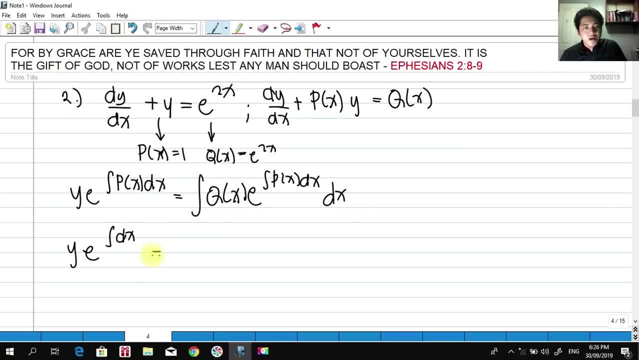 So this is simply integral of dx, now equal to the integral of q of x. e raised to 2x Multiplied by e raised to the integral of p of x is 1, So this is simply dx and we have dx here. So that is y, e raised to x, because the integral of dx is x. 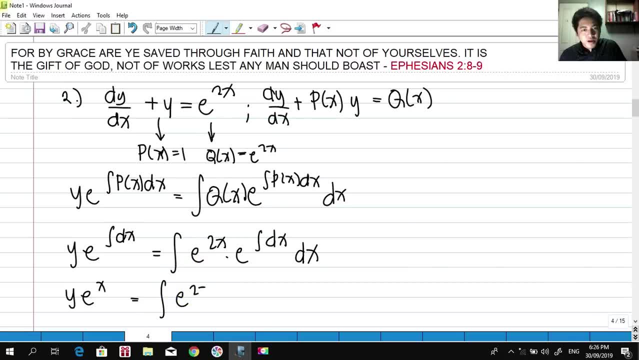 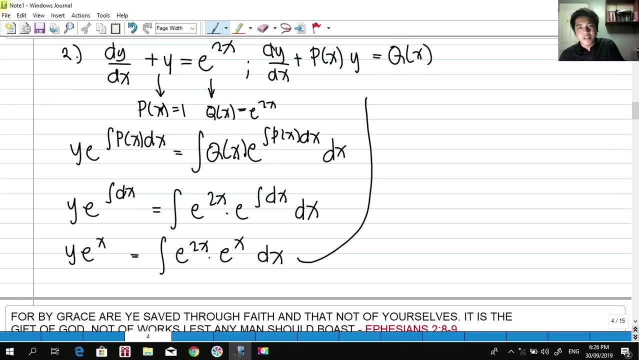 Is equal to the integral of e raised to 2x multiplied by e raised to x. Okay, Okay, And we have dx here And, as you can see, by laws of exponent These two have the same base, So we can rewrite this as Y. e raised to x is equal now to: 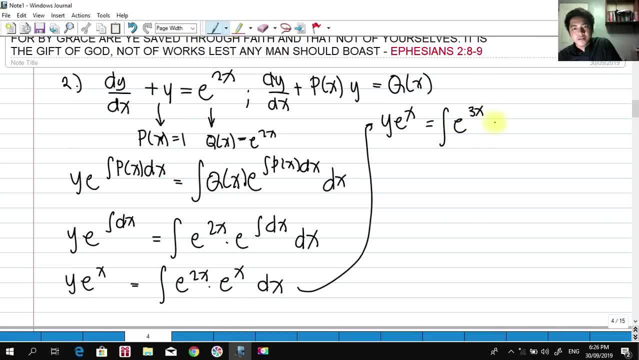 Integral of e raised to 3x to dx. So if we evaluate the integral on the right side of our equation, We have 1 third e raised to 3x plus c. Okay, So So, And if we're going to simplify this, This can be the answer. 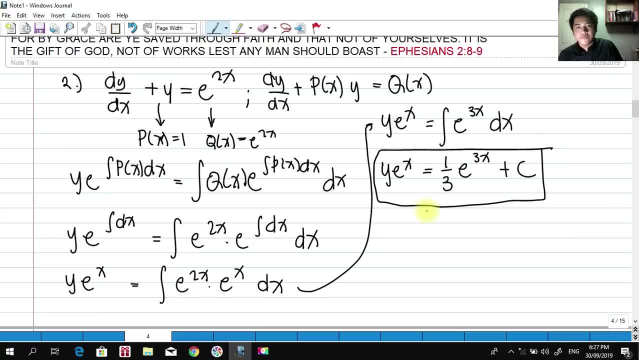 But if we're going to simplify this, Okay. Furthermore, If we're going to express this in terms of, only in terms of y, We have e raised to 3x over 3 e raised to x. I've divided the whole equation by e raised to x. 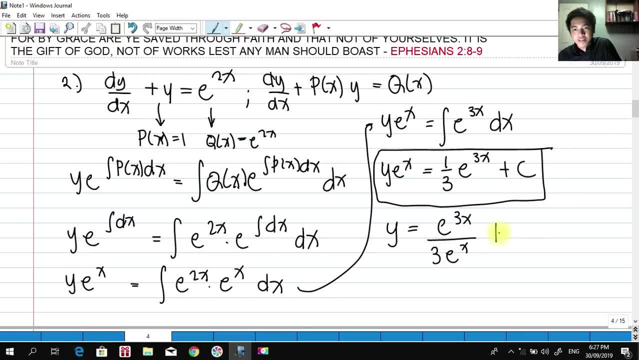 Just to eliminate the e raised to x here. So we have plus c over e raised to x. As you can see by properties of exponent: e raised to 3x divided by e raised to 3x. So we have e raised to 3x divided by e raised to 3x. 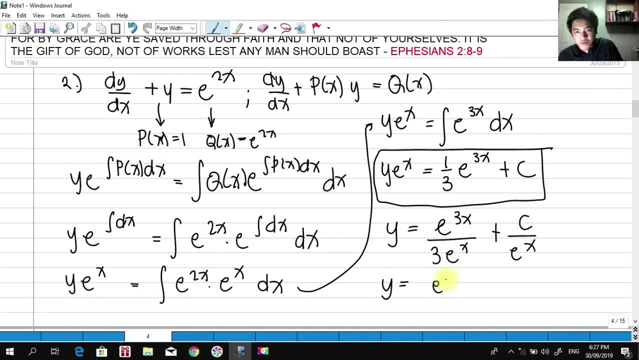 So we also have e raised to x. That should be: y is equal to e raised to 2x over 3 Plus this. I can This e raised to x. I can put this on the numerator Such that it would have a negative exponent. So this should be our answer. 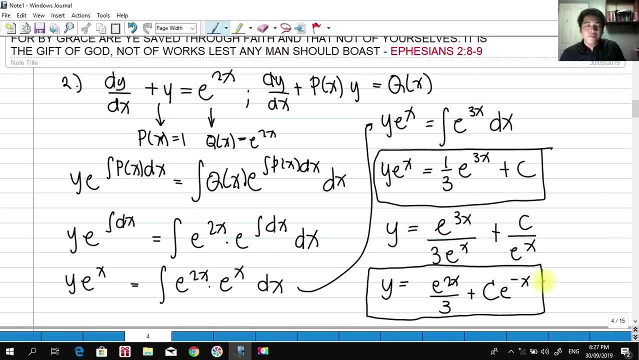 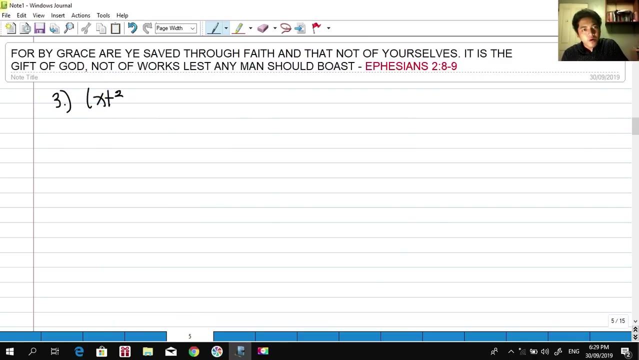 Okay, So we did nothing special here, But we apply our knowledge in our algebra. Okay, so by x, loss of exponents, okay, and of course the integral. so again another example, so that we can practice our skills in solving. so we have x plus 3y, dx minus x, dy is equal to 0.. now, this type of differential equation we cannot actually see. 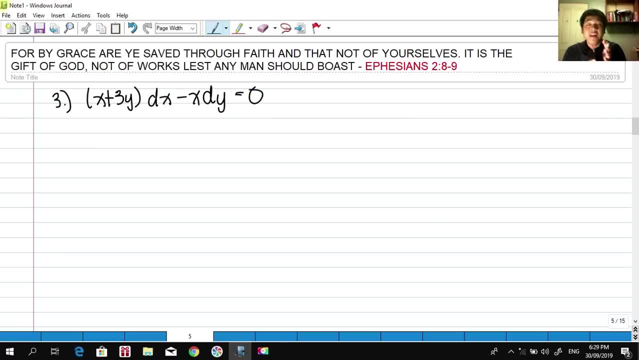 whether it is dependent in y or linear in y- i'm sorry- or linear in x, unless we distribute this. so we have x, dx plus 3y. dx is minus x, dy is equals to zero. so the thing here is clear. okay, here is the secret. if, if the dx or the dy, you're going to look at the dx and 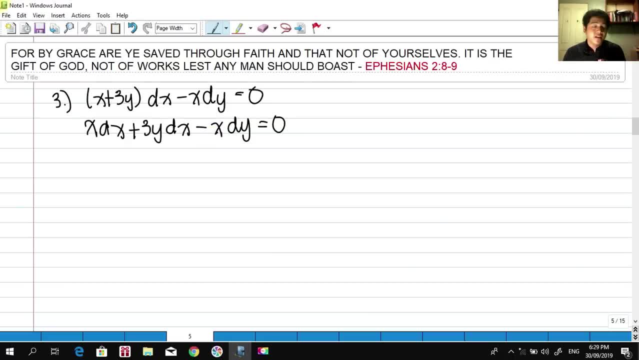 the dy? definitely, because that is the dy over dx or dx over dy. so that would depend on what is the linearity of this d. is it linear in x or linear in y? so if the dx has a greater term, okay, we have two terms of dx here: x, ds plus dy dx. then that is not linear in x. but if we see 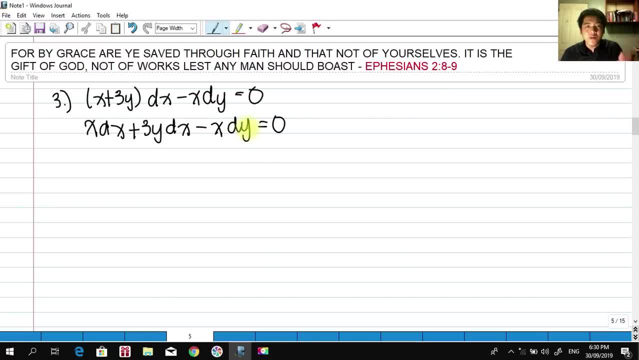 okay, only one term. with dy, then that is the linearity of our de. okay, that is linear in y. so if we're going to transpose this on the other side, we have x, dy minus x, dx minus 3 y. dx is equals to zero. so if i'm going to divide this both by, so what will happen here is that we have we. 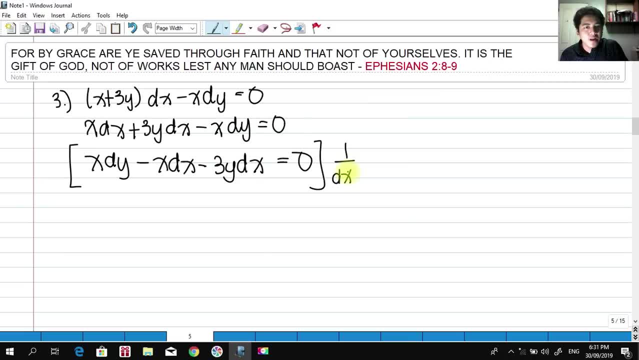 divide this by dx. okay. so what will happen? we have x dy over dx, minus x, minus dy over dx. so this is a linear fried eine hyd Yazik d1, y is equal to zero, and if i'm going to further transpose this x on the other side of the equation, we have this equation, okay and actually. 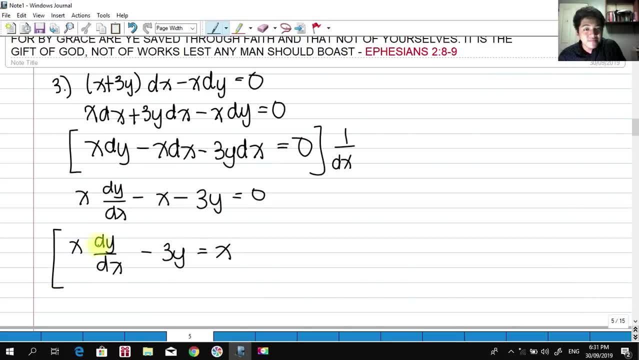 i still have to eliminate, i'm sorry, x here for this dy over dx to be left alone on this side on this term. so what will happen? we divided by one over x, so we have dy over dx minus team equals d. i over dx equal 0, so x. this will end here. what will happen here is we have this d, this one here. 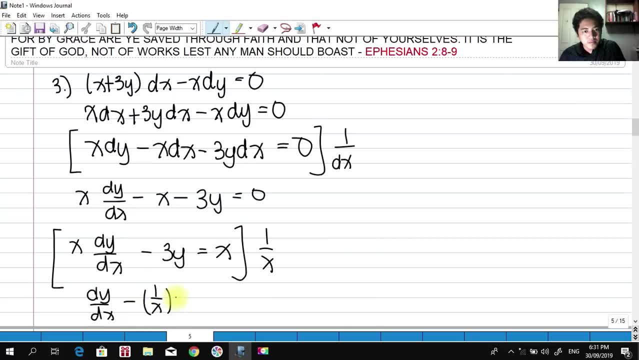 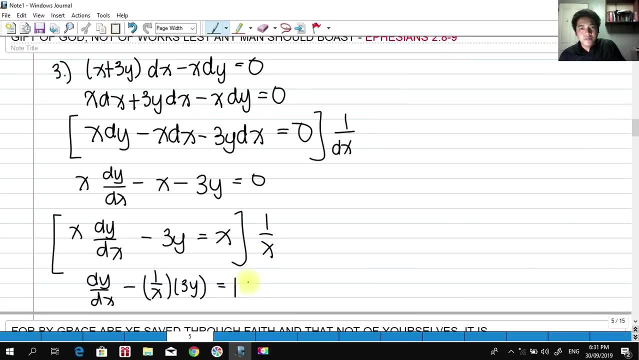 d y over dx minus x. y is equal to negative enemy t minus. we came up with two terms, so we have d y over♪ x minus 1 over x multiplied by 3y is equal to 1.. Or, of course, we have dy over dx minus 3 over x multiplied by 1 is equal to 1.. 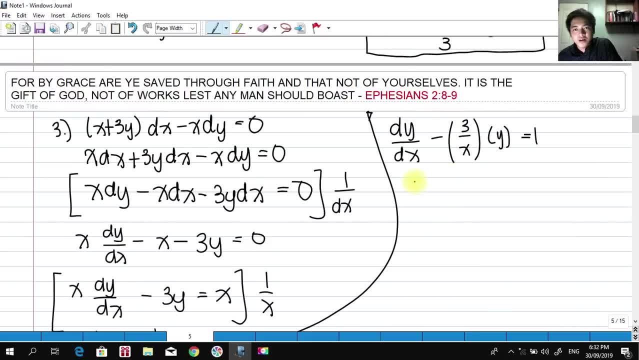 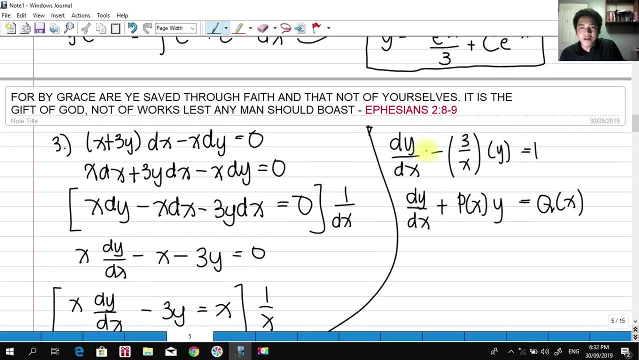 Why? Why did I get the 3 here? Because our formula, our form for linear in y is dy over dx, p of x multiplied only by y. So I have to isolate y here is equal to q of x. So now we have our dE written in linear in y in the form of linear y. 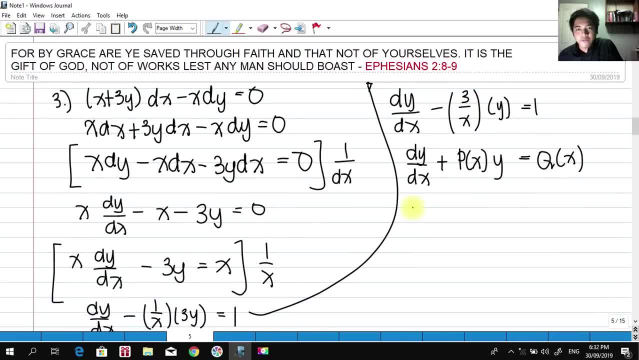 So what will happen here? is that okay? we apply the formula again: y. e raised to integral of p of x, dx is equal to integral of q of x. e raised to the integral of p of x, dx and dx here Wherein our p of x here. is this okay? 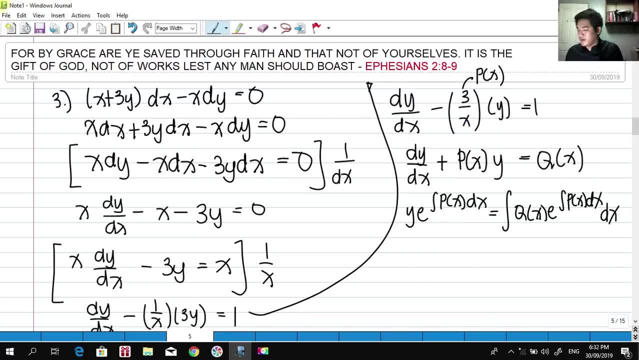 Our negative 3 over x here. okay, So we simply substitute. By the way, this is our q of x, the 1 here. So q of x can be 1, right, It can be a constant, Because we have written already the dx. 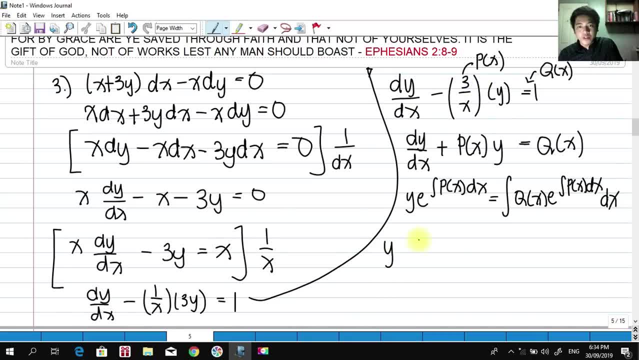 So we have y multiplied by e, raised to the integral of negative 3 over x, That is, our p of x, including the negative. dx is equal now to the integral of q of x, which is 1 multiplied by e raised to negative 3 of x dx. 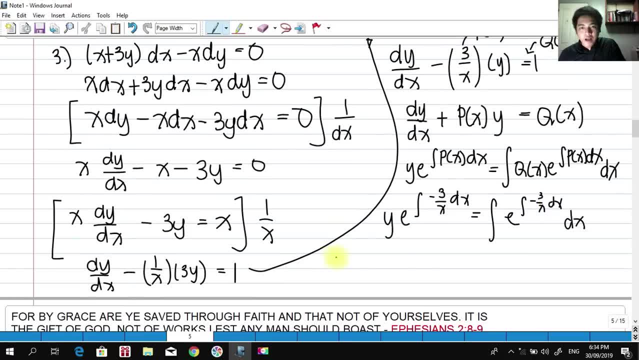 We have dx here. okay, So to evaluate, we have y- e. If I evaluate this integral, we can factor out Negative 3 outside of the integral. we are left with dx over x here, And the same way goes here. 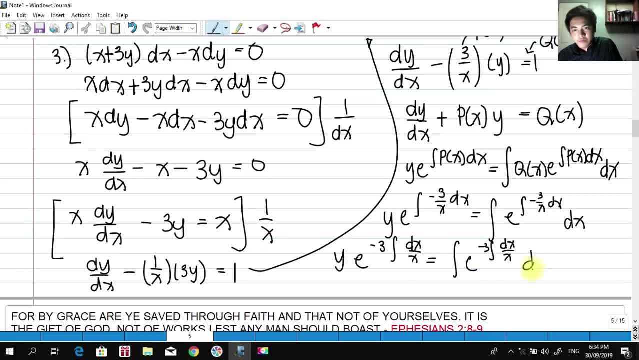 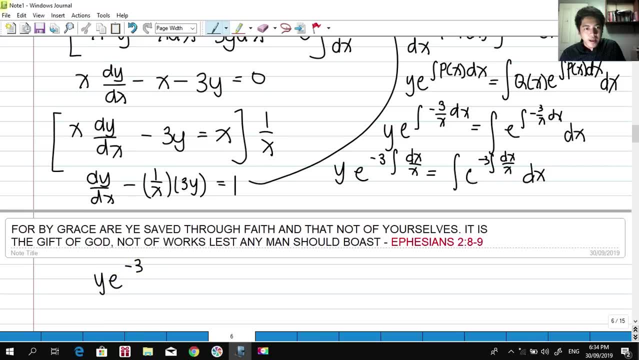 We have negative 3.. We have dx over dx here and we have dx here. So what will happen? if we evaluate that We have y multiplied by e raised to negative, 3 ln of x is now equal to the integral of e raised to negative 3 ln of x. 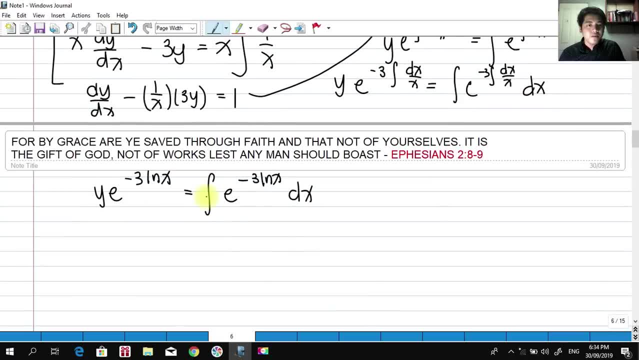 and dx here. okay, My properties of natural logarithm. we can rewrite this as y, e raised to whatever constant inside of the ln. we can make this the exponent of the inside function of the ln. So we have ln of x raised to negative 3, and that goes the same for this integral. 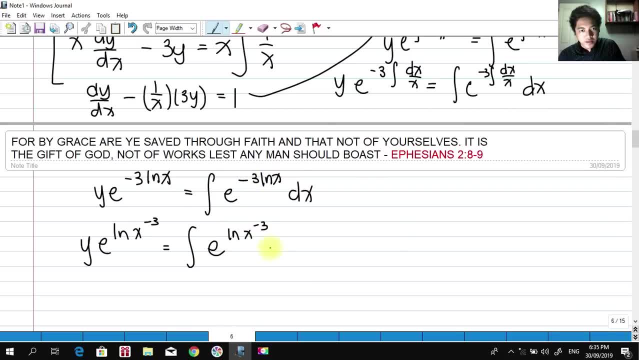 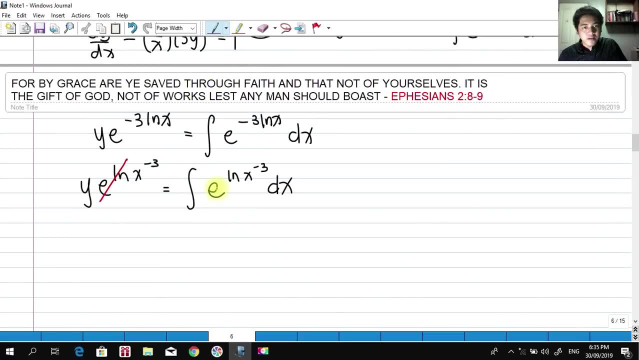 We have e raised to ln, x raised to negative 3, we have dx, So we can cancel out Of course. Of course e raised to ln, e raised to ln here, and then we're going to get y multiplied by x raised to negative 3 and this is now the integral of x raised to negative 3, dx. 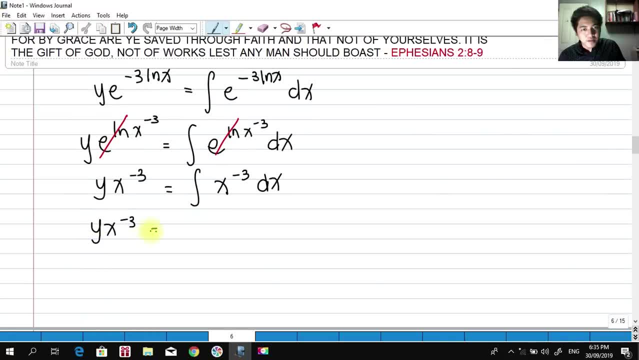 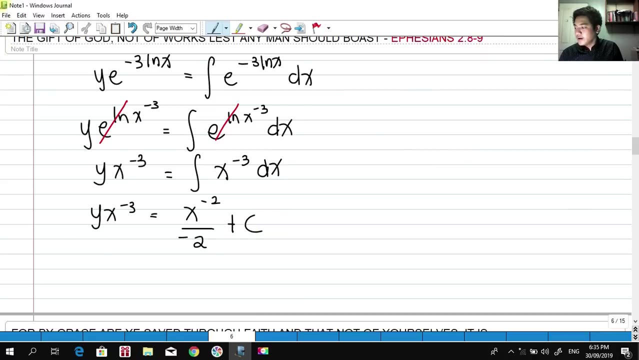 Evaluating the integral, we have y, x raised to negative 3.. We have x negative 3 plus 1, that's negative 2 over negative 2 here plus c. alright, And if we're going Again to at least somehow get the simplification of this, okay, the simplification of this. 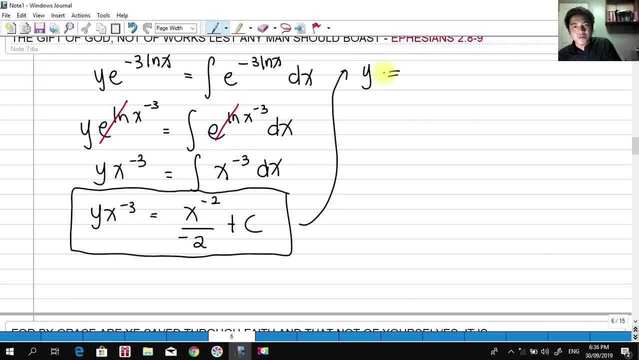 we can still. we have: y is equal to x raised to negative 2 over negative 2, x raised to negative 3 plus c over x raised to negative 3.. And if I'm going, Let's see, Let's see If I'm going to apply the rules of exponent we have. well, let's say I'm going to pop. 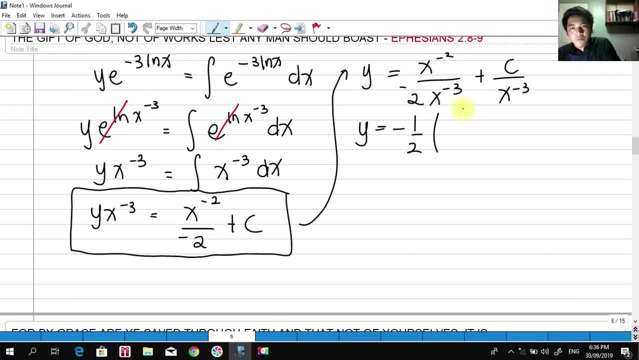 out negative 1 half first. So that is multiplied by 1 over. I can bring this down: x squared multiplied by x, okay, x negative 3 here. okay. So plus c over x raised to negative 3 here. So what will happen is that we have y. 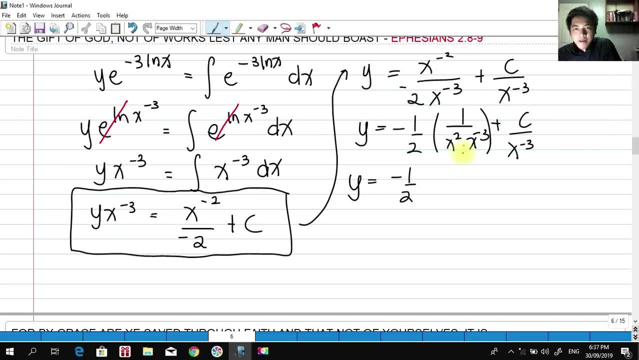 Okay, Y is equal to negative 1 half and by law of self exponent we can add the exponent, so 2 plus negative 3, that should be 1 over x raised to negative 1, negative 3 plus 2 is: 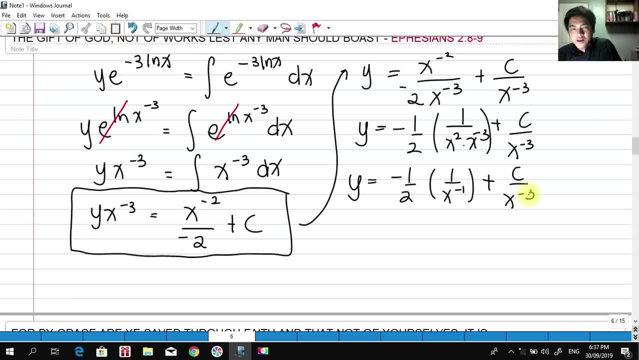 negative 1, plus c over x raised to negative 3.. And furthermore we have: y is equal to negative 1, half of x. okay, plus c, x cubed. This is also an acceptable answer. Okay, And of course, some problems. even books, okay, leave the other side of the equation. 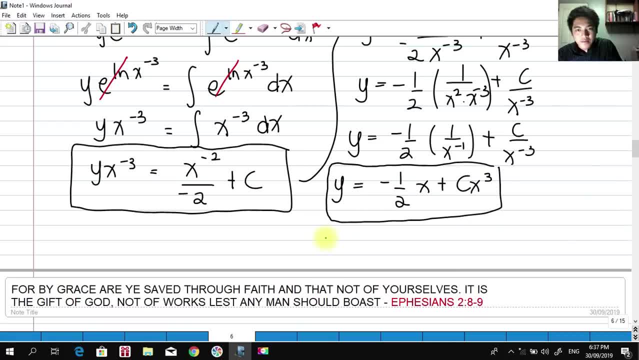 as c. So another possible answer is that we have: 2y is equal to negative x. If I'm going to multiply both sides of the equation by 2, notice that this c would still not be affected because it has a constant here. 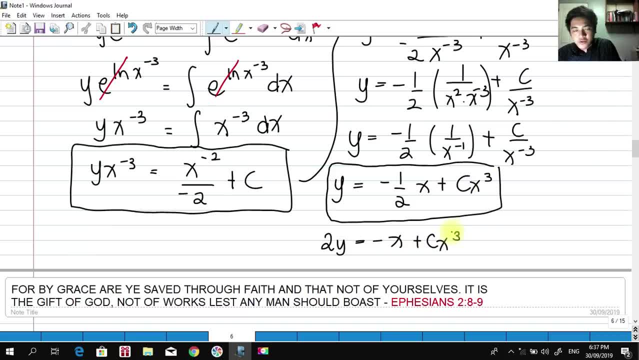 So we have negative x plus c x cubed here. Okay, In terms of c x cubed we have. Okay. So negative x cubed here is equal now to 2y plus x. This is another acceptable answer, Okay. 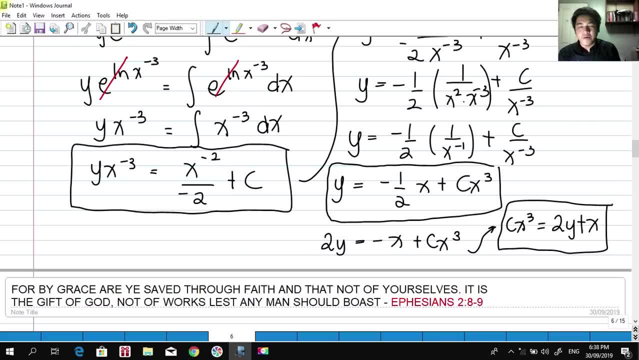 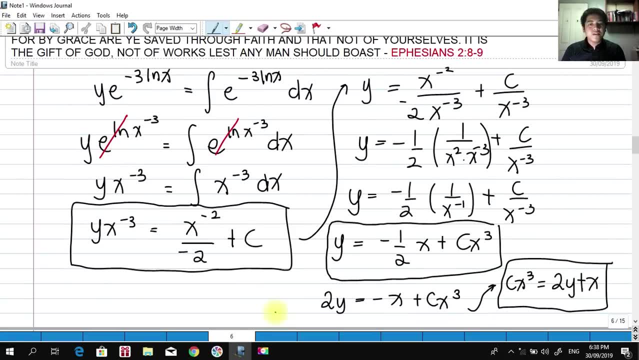 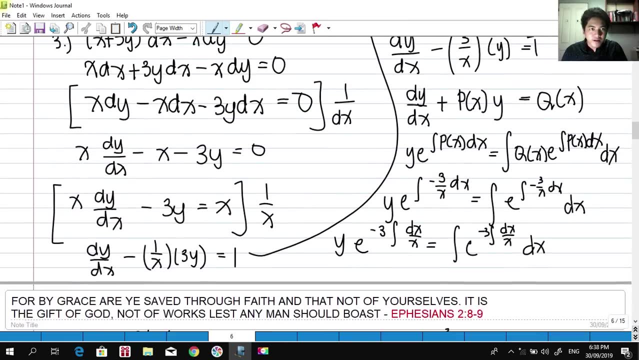 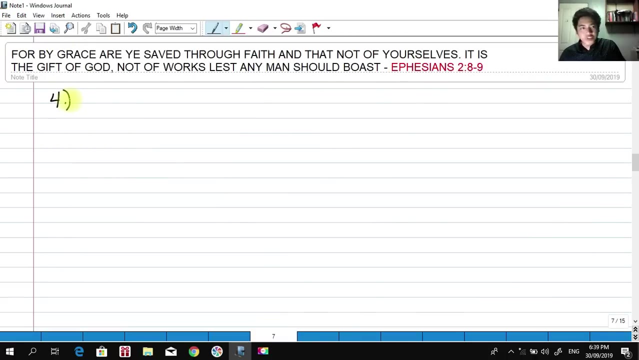 So that is, that is the answer for our DE. Okay, Let's try to solve again problems. So for how? for what problem is it right now? For problem number four, Four, Four. we have the given which is y, dx plus 3x minus xy plus 2dy is equal to 0. 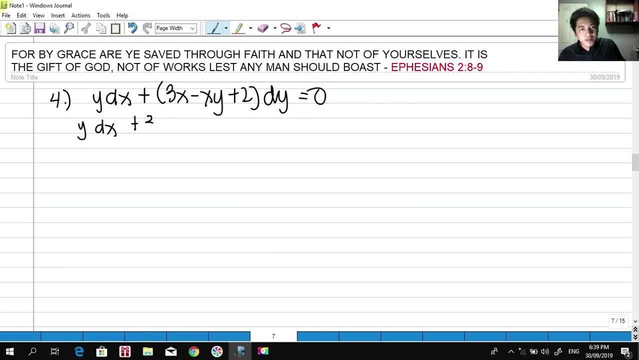 If I'm going to distribute this y, dx plus 3x, dy minus x, y, dy plus 2dy, as you can see here. okay, you have already an idea that this is a linear in xy, Because we have only one term in terms of x. 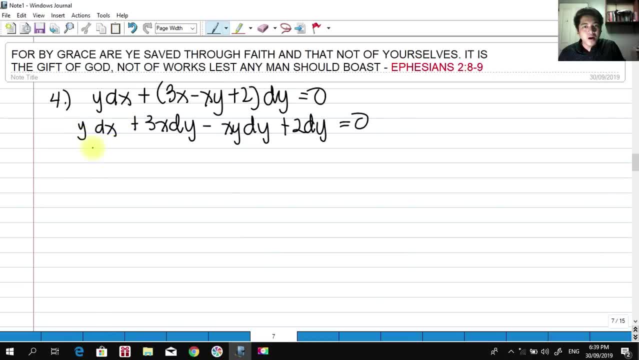 Okay. So if I'm going to to actually rearrange this, furthermore, we have y, dx, Okay. Plus, can I factor out x in here? So we can factor out x in here. So we have okay x multiplied by. I can factor out also dy x multiplied by 3 minus y dy. 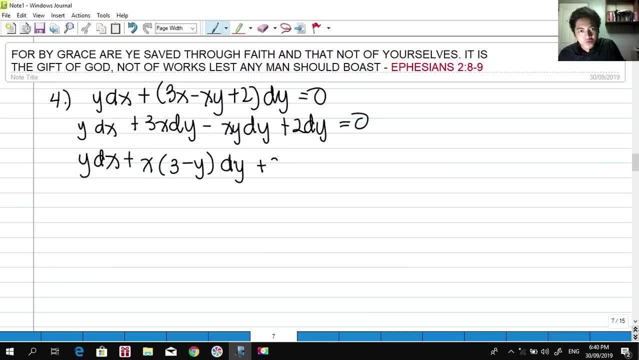 Okay, Plus 2dy is equal to 0. Okay, So, furthermore, y dx plus x times 3 minus y dy is equal to negative 2dy. Agree, And if I'm going, if this is linear in x, remember that our formula for linear in x, 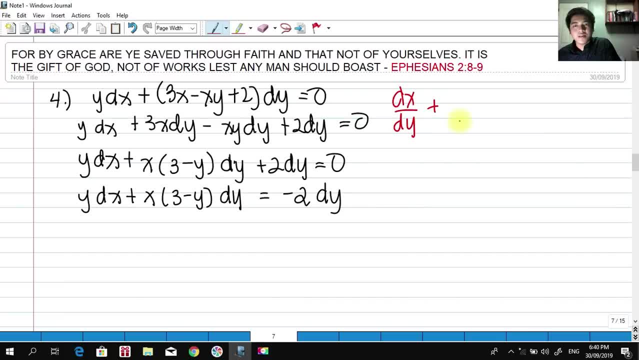 is dx over dy plus we have p of y multiplied by x. Okay, Is equals to the p of y. So if I'm going to multiply both sides of the equation such that I'm going to eliminate y here and I'm going to add or to have dy here, 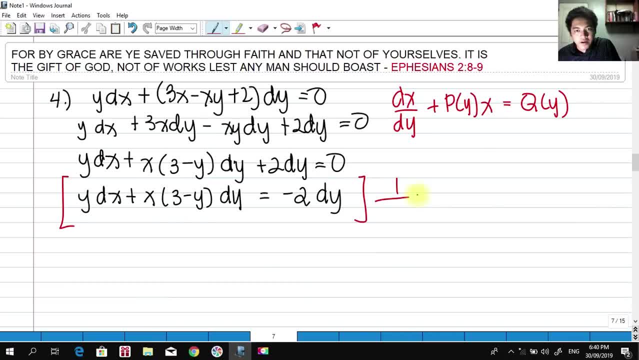 So what will happen is 1 over. I'm going to eliminate y here. We have a y here, Okay, And multiply it by dy, So it has to cancel dy's here. So what will happen is that we have dx times dy. 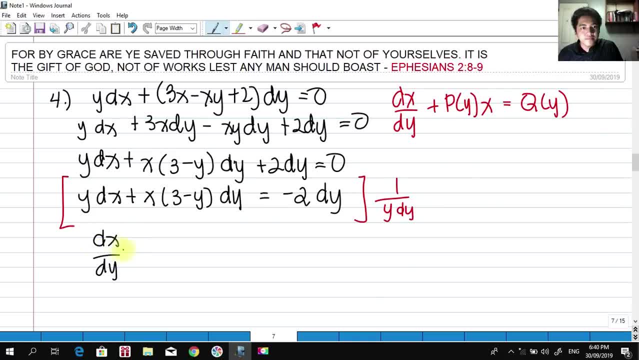 We have dx over dy plus okay, plus dy's will cancel here. So we have x multiplied by 3 minus y over y. Okay Is equals to: again dy's will cancel negative 2 over y. As you can see here class that we have transformed this d into a linear form. 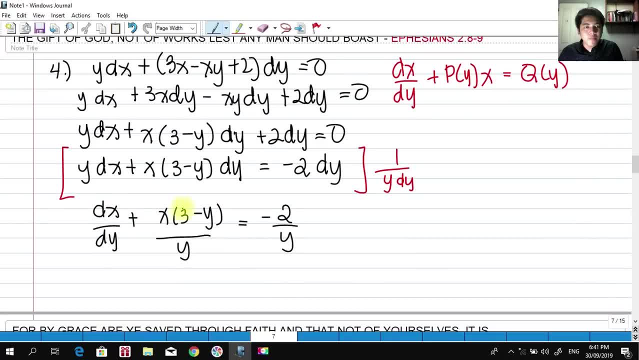 Whereas, okay, If we're going to separate x here, this is separated already. x, That is our x, This is our p of y, as you can see purely in terms of y, And this is our q of y. 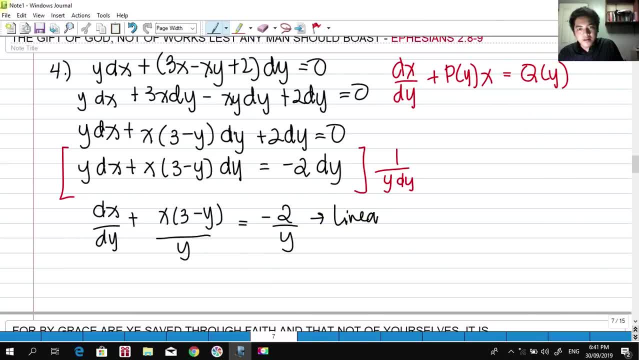 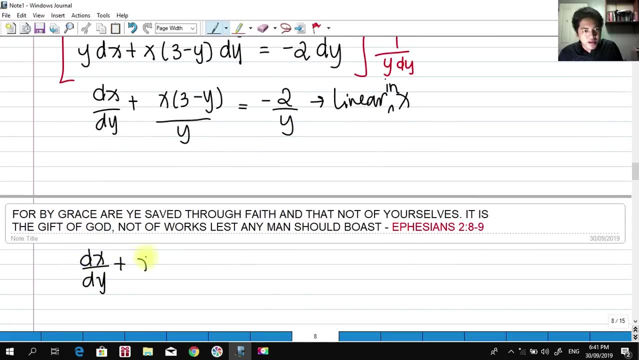 So hence that is linear. again, linear in what? In the dependent variable x? Linear, oops, in x. Okay, So let me just rewrite this so that we have enough space: dx over dy plus x, multiplied by 3 minus y over y is equals to negative 2 over y. 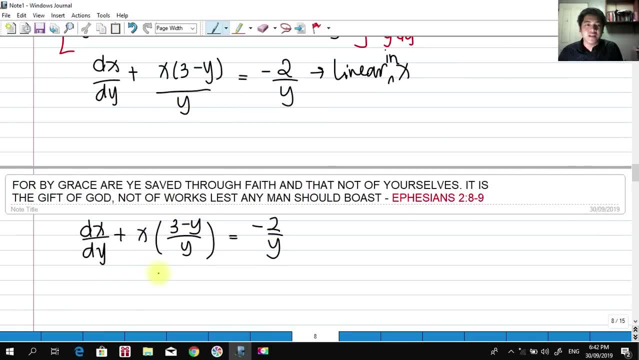 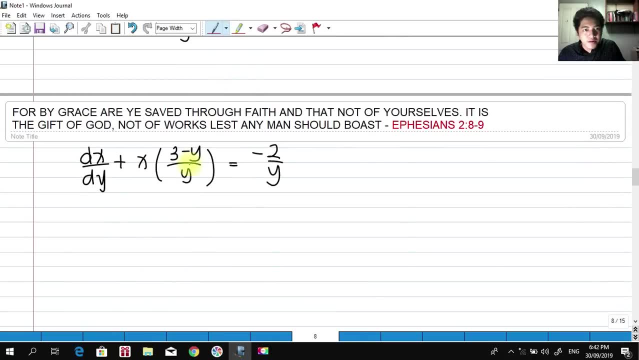 So this is the same as this. I only factor out x because that is our x term. So this should be our 3 minus y over. y should be our p of y And this should be our q of y. Okay, And furthermore, 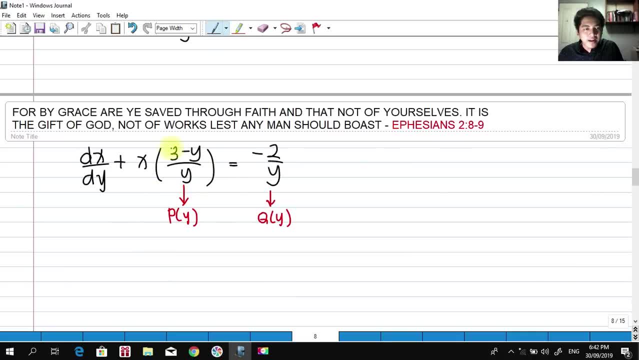 If I'm going to rearrange this, okay, so that it's easier for us to integrate this, because we're going to integrate this Okay. Remember, we're going to integrate this because e raised to integral of py, dy, So plus x. 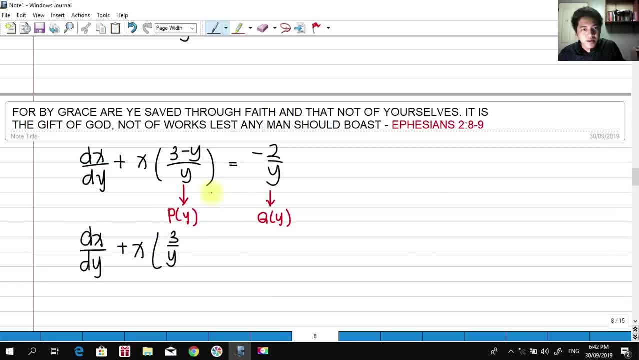 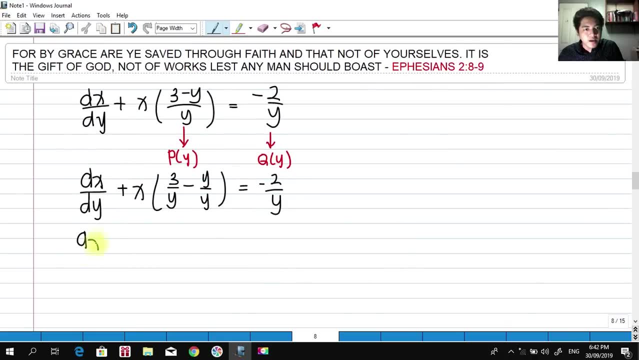 If I'm going to simplify this, that is, 3 over y, minus y over y is equals to negative 2 over y. So if I'm going to simplify: dx over dy plus x, multiplied by 3 over y minus 1, right is equals to negative 2 over 1.. 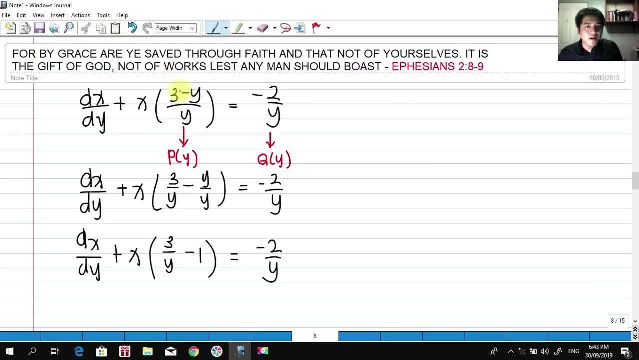 So I've distributed the negative here, okay, such that this can be rewritten as this: Okay, So you can see, y's will cancel, will give you 1.. Okay, So this is our p of y and this is our q of y. 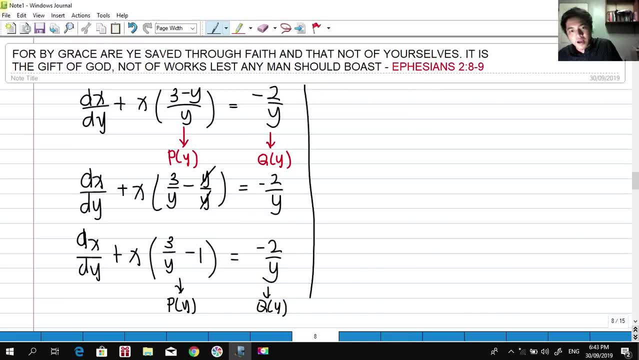 And again, If we're going to recall what is the formula, if that is a linear, next, that is: x multiplied by e, integral of p of y, dy is equals to integral of q of y multiplied by e raised to p, integral of p of y, dy and dy. here, 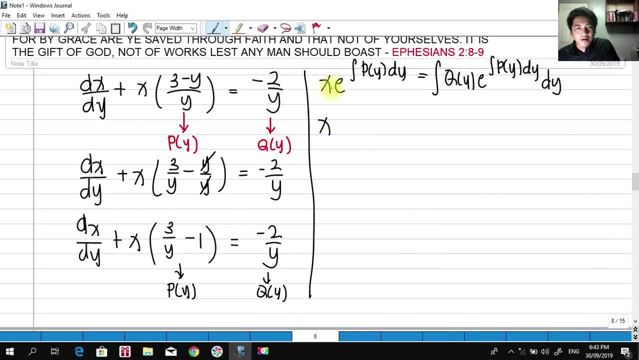 Our x is simply x. Okay, That is our dependent variable. multiplied by e Integral of p of y, That is 3 over y minus 1 dy, is equal now to the integral of q of y, that is negative, 2 over y. multiplied by e, raised to the integral of p of y, which is 3 over y, minus y, 1 dy, and: 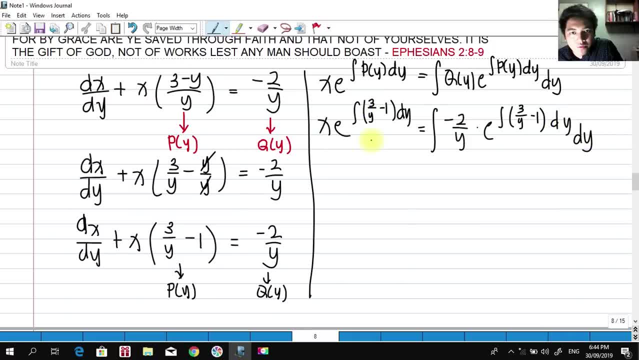 we have dy. Okay, Notice, if we're going to first- okay, evaluate this, Let's evaluate the integral. Okay, We're going to first evaluate the integral for you: 3 over y minus 1 dy. We can separate the integral sign and the dy. 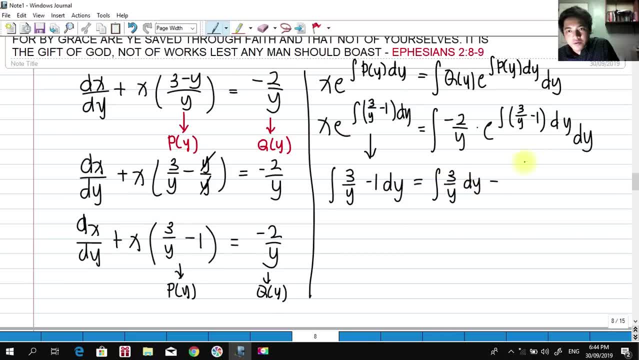 So we have integral of 3y dy minus 1.. Okay, That is equivalent to dy. So I can factor out 3 outside the integral sign. We have dy over y here minus the integral of dy. So you can see we can integrate this. 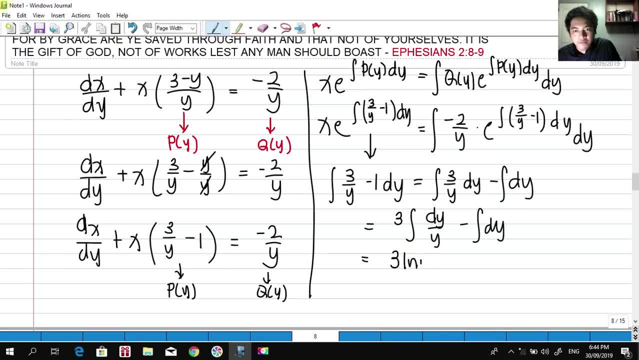 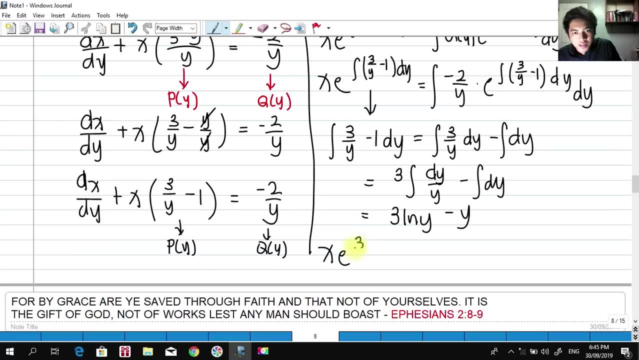 So we have dy over y is 3ln of y minus y. Okay, And if we're going to, this is only the exponent of the e here. So we have evaluated. So if I'm going to rewrite, that is x e raised to 3ln of y minus y. 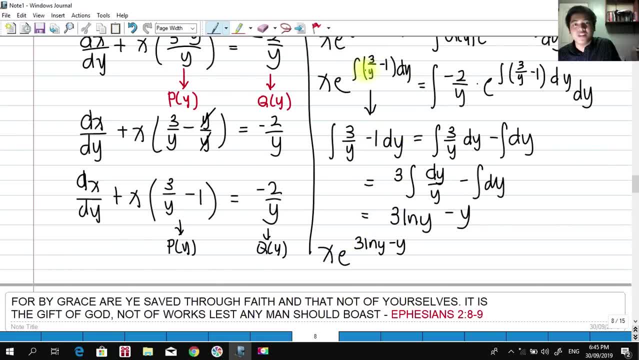 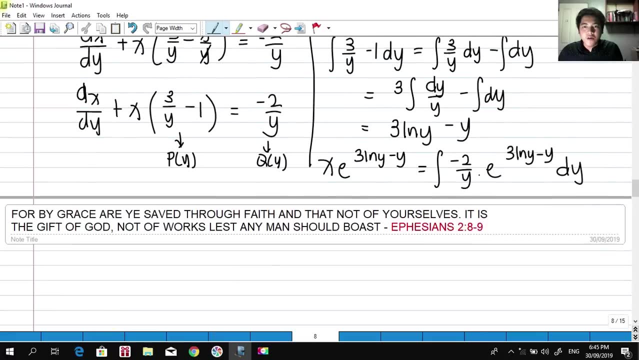 That is the evaluated integral we evaluated a while ago. That is only the exponent of e is now equal to the integral of negative 2 over y multiplied by e, raised to 3ln of y minus y dy. Okay, So we should simplify this first. 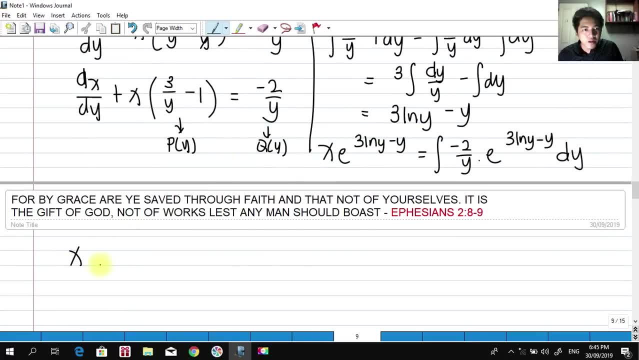 We know that by properties of exponent we can derive e raised to 3ln of y minus 1 as e raised to 3ln of y minus e Okay, Minus e Okay, Raised to y Okay. We can rewrite this at that form. 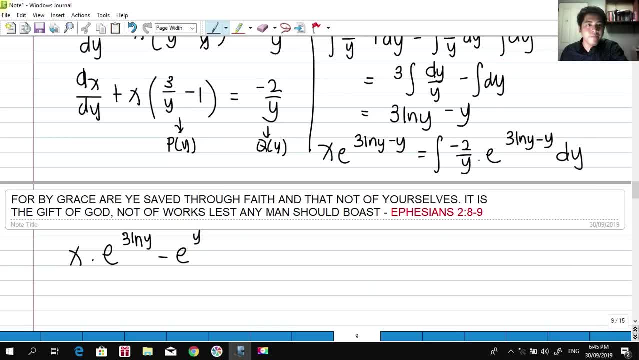 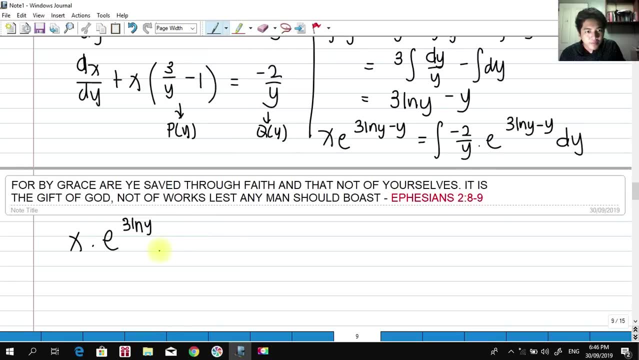 Okay, Oops, I'm sorry. This is not this, but rather this is multiplied by e raised to negative y, because we have this form. So this is the loss of exponent e raised to 3ln of y minus y can be rewritten as this: 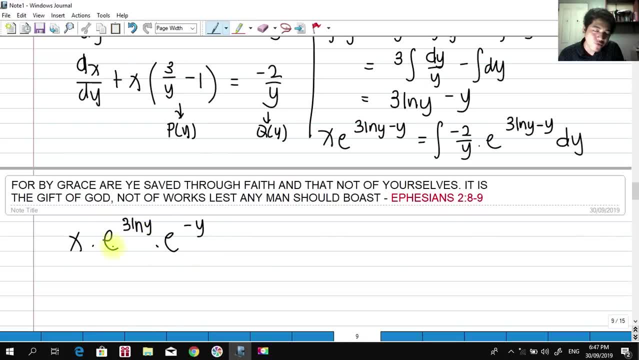 Okay. So because if we have two bases here, we can definitely add: Okay, Since this is negative, it results to minus. So, okay, This is a multiplication, We can add exponents, But we did the reverse thing. Okay, So this can be rewritten by loss of exponent, as this: 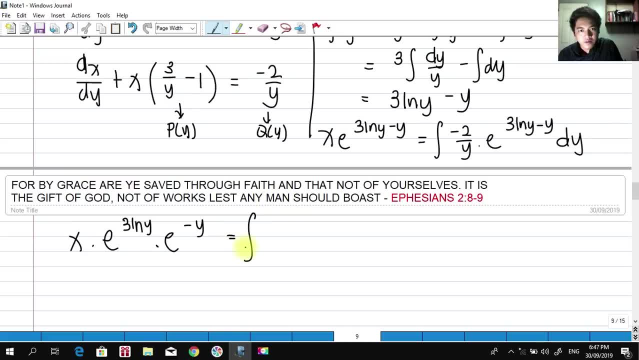 And that is equivalent to now, negative 2 over y. The same thing I will do here: E multiplied by e raised to 3ln of y multiplied by e raised to negative y dy here. So, as you can see, applying the properties of the expression, we can see that we can add. 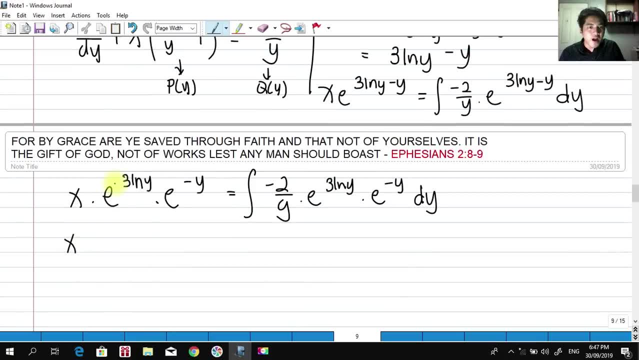 exponents We can see applying the properties of natural logarithms and we have ex times: e raised to ln of y cubed multiplied by e raised to negative y is now equal to negative 2 over y. The same E raised to ln of y cubed multiplied by e raised to negative y dy. 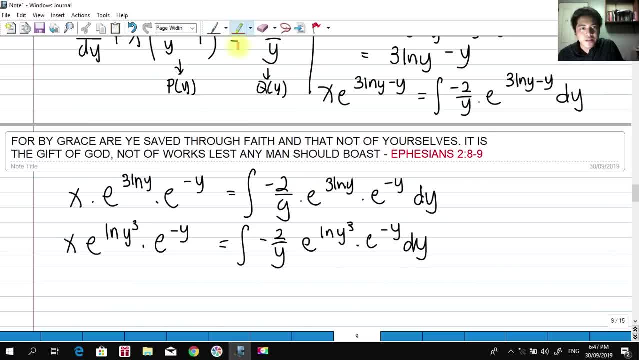 And as you can see here- Okay, So you can see here- This e raised to ln will cancel And we are left. We are left with x y cubed, e raised to negative y here, And we are left with the integral of negative 2 y here as over y y cubed multiplied by e. 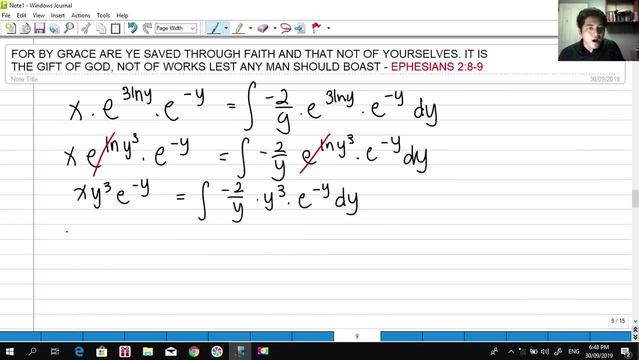 raised to negative y dy. So I can factor out on the right side of our equation the negative 2 integral of y cubed over y. That is a multiplication multiplied by e raised to negative y dy in here. So we can see that this will cancel. 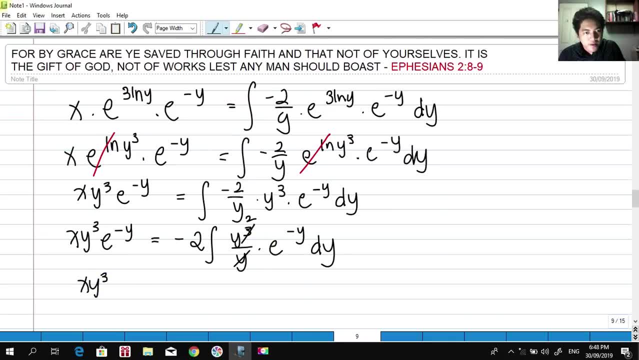 This should be y squared. So we have x- y cubed multiplied by e raised to negative y. We have negative 2 integral of y squared multiplied by e raised to negative y, dy. And this is an integration by parts. So, as you can see, 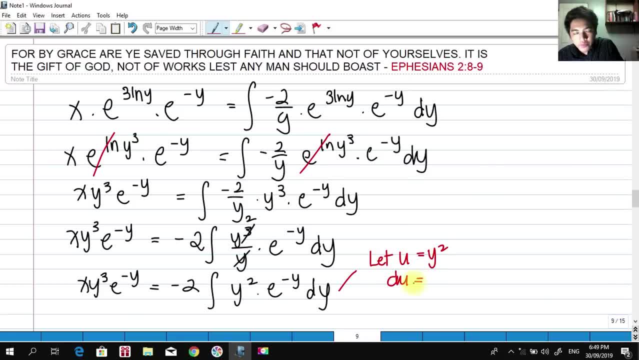 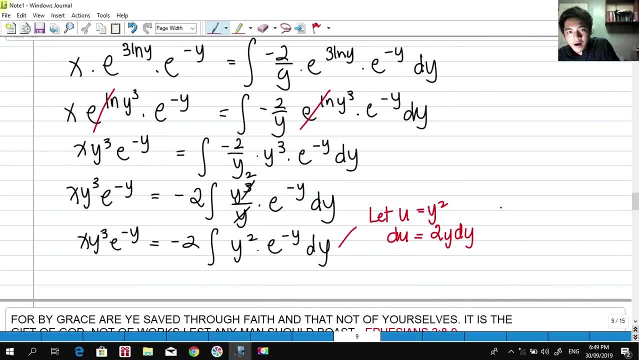 We can left u as y squared du with respect to y is 2 y dy, Integration by parts, And we left dv as what e raised to negative y dy And we let v. We evaluate the integral of this. That should be what. 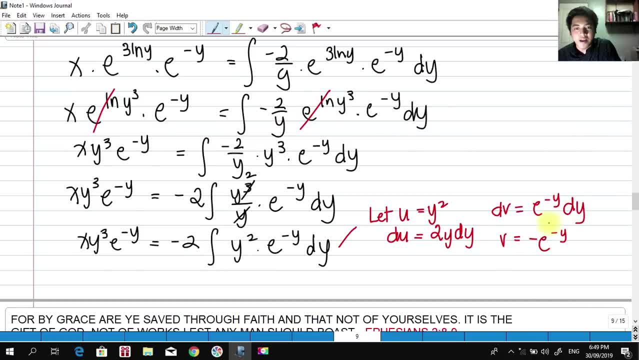 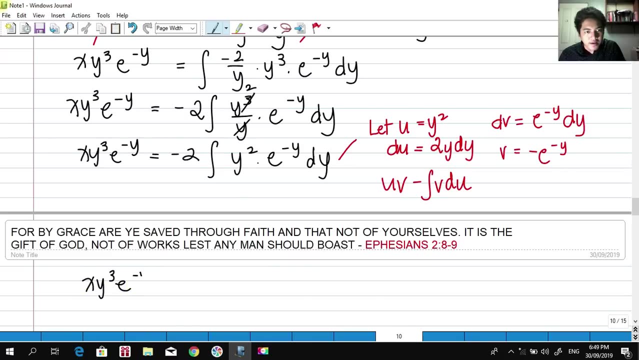 Negative e raised to negative y. Yeah, That is the d, And the formula for integration by parts is again ub minus the integral of vdu. Okay, So we should learn, or we should have learned, this in our integral calculus course. So negative 2 multiplied by ub minus vdu. 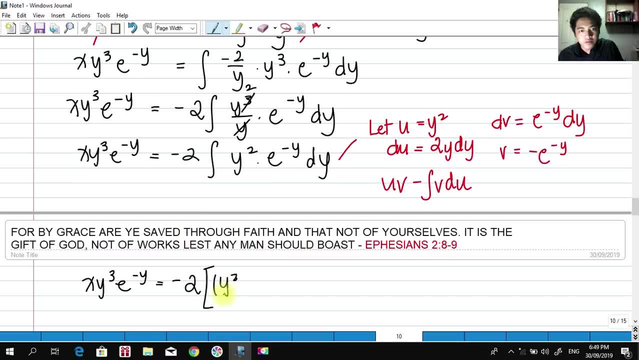 Our u is y squared, y squared multiplied by v Negative e raised to negative y, Minus the integral of v Negative e raised to negative y du. Our du is 2 y dy. Okay, So, upon simplifying, We have: 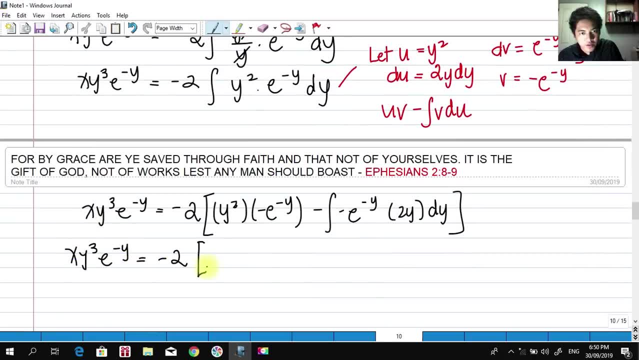 Okay, First, negative 2.. Negative e raised to negative y, y squared. Okay, We can factor out 2.. Because it is a constant And the negative sign here, So negative 2.. We can factor out negative 2.. 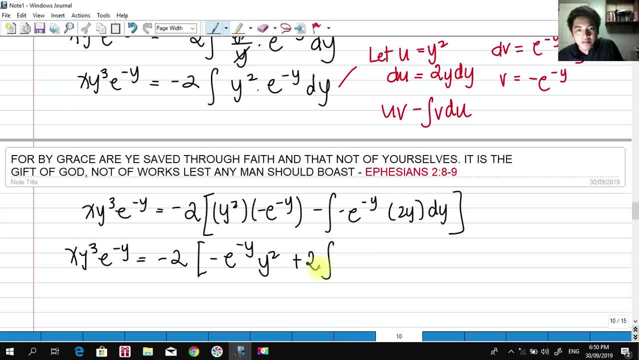 And this is a minus, So that becomes 2.. Integral of e raised to negative y, Multiplied by y, dy, And again, Again, Again, We have to distribute negative 2 here. Okay, So we have positive 2 y squared. 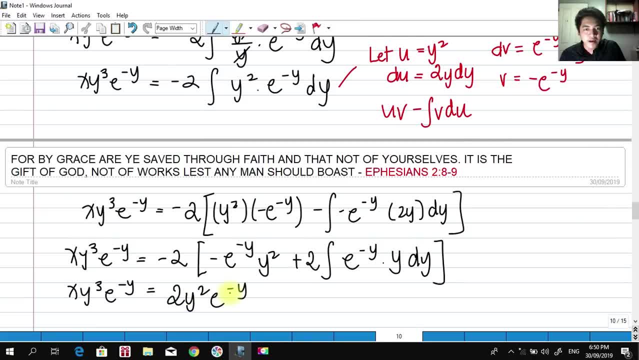 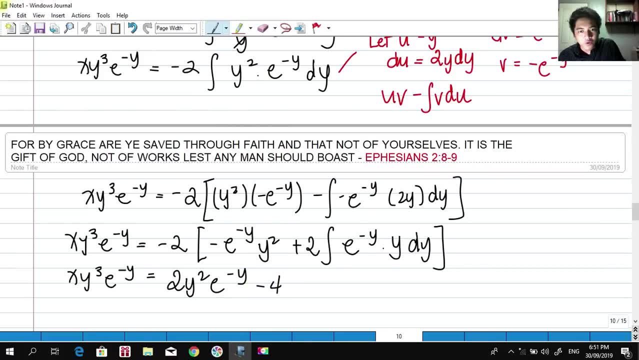 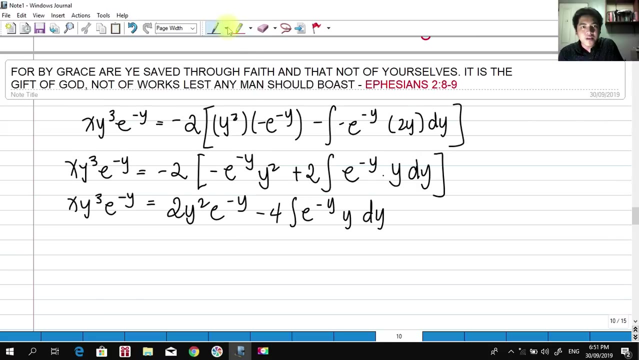 e raised to negative, y Okay, Plus or Sorry. Negative 2 times 2 would be minus 4.. The integral of e raised to negative, y Okay, Multiplied By y dy, And, as you can see, We are going to get the integral again of this. 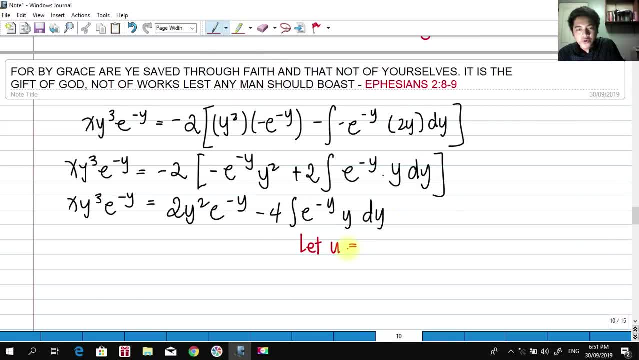 That is again integration by parts. So we have to let u equal now to y. Derivative of u with respect to y is dy. Our dv now would be: e raised to negative y dy, Still the same, Our v. We get the integral of this. 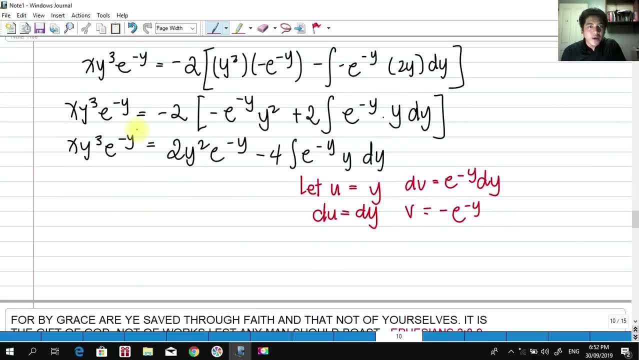 Negative e raised to negative 1.. So, Upon continuation of our solution here, We have xy cube. e raised to negative y is equal to 2y squared. e raised to negative y Minus 4.. Multiplied by the integral of this: 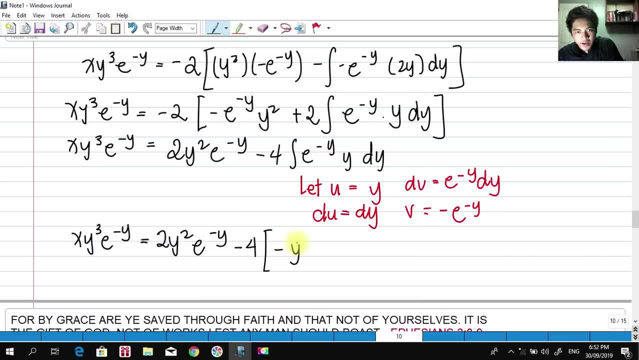 That is uv minus vdu. We have Negative y e raised to negative y. Okay, That is u times v Minus the integral of vdu: negative e raised to negative y. Then we have- Finally, We have dy here. 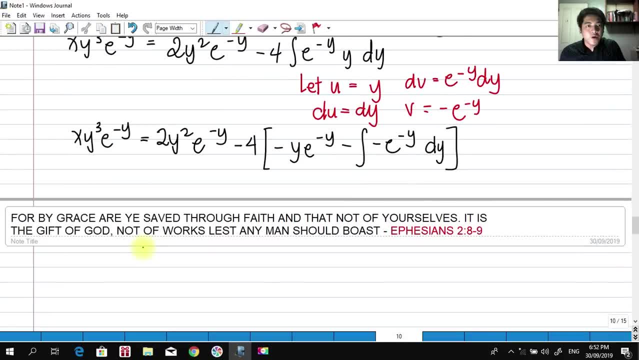 Because du is equivalent to y. So, Upon simplifying, We have xy cube. e raised to negative y Is equal to 2y squared e raised to negative y. Okay, If I am going to simplify First This: 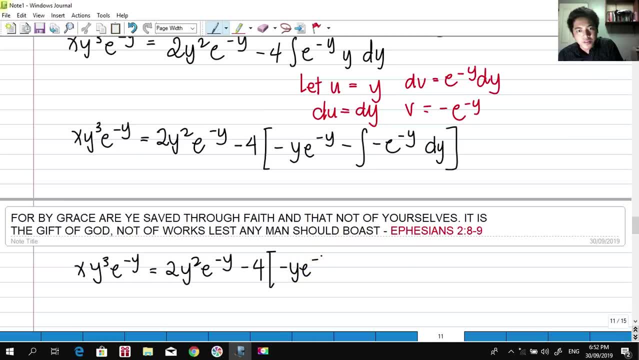 I can, What I can factor out: Negative sign Outside the integral sign. So Minus negative That becomes Positive The integral of e raised to negative y dy. And If we are going to distribute The integral of e raised to negative y. 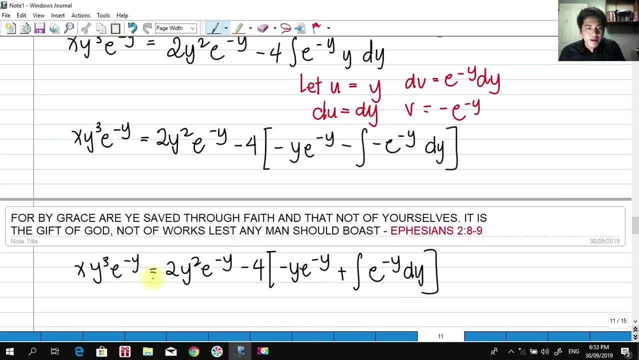 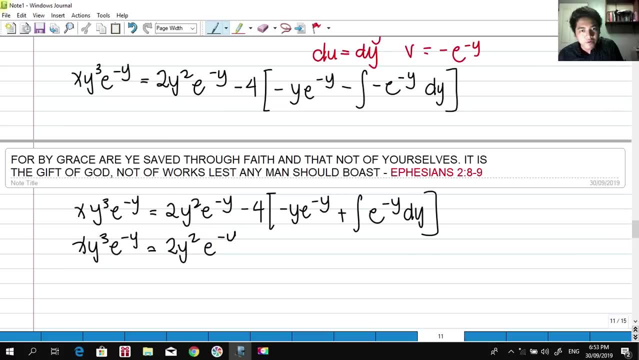 dy, And If we are going to distribute The integral of e raised to negative y dy, And If we are going to distribute The Negative 4 term here Or The constant negative 4 term 4 here. 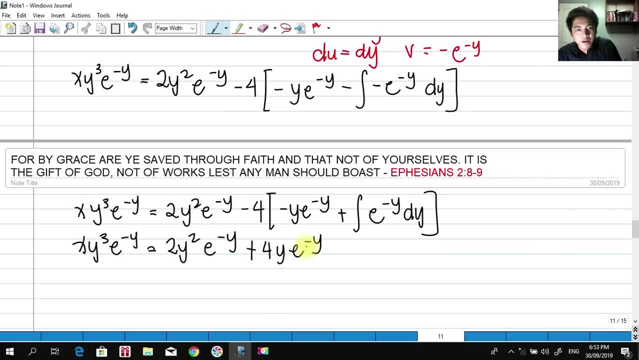 So That becomes Plus 4y. e raised to negative y And This is Minus 4.. The integral Of e raised to negative y Is negative e raised to negative y. Don't forget The plus. 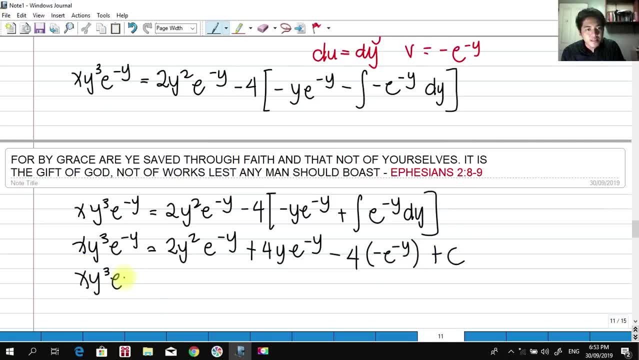 c. So If we rewrite this, We have 2y squared e raised to negative y Plus 4y e raised to negative y Plus 4y e raised to negative y Negative 4. Multiplied: 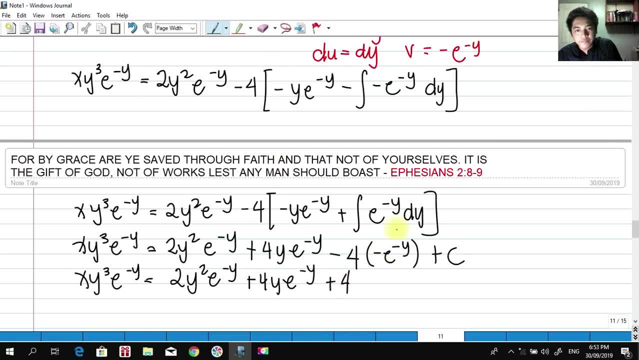 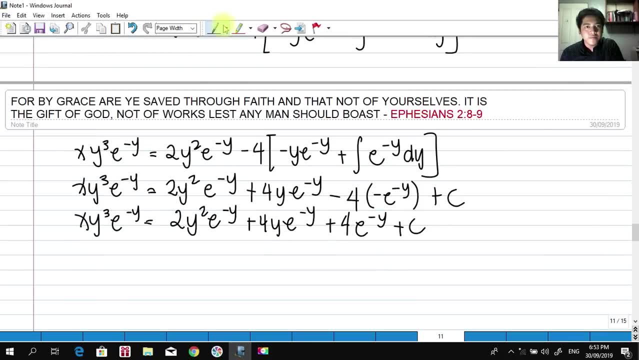 By this negative, That should become Plus 4.. e raised to negative, y Plus c. Okay, And As you can see here, Okay, We can multiply This Full equation Or Simplification By: 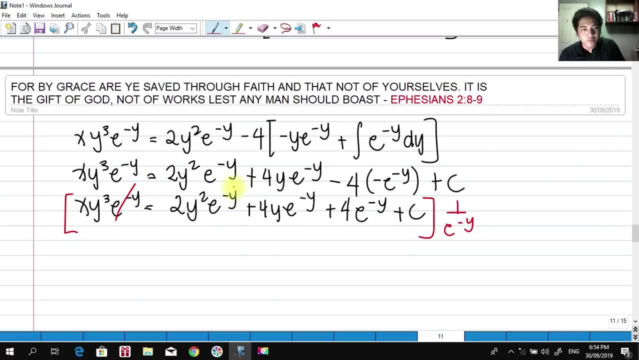 1 over e raised to negative y. So That what will happen? Our e raised to negative y Here Will cancel, Okay, And Our term of c, Okay. We will be having This 2y squared. 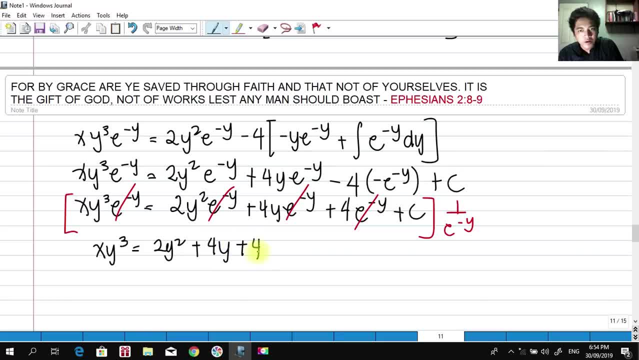 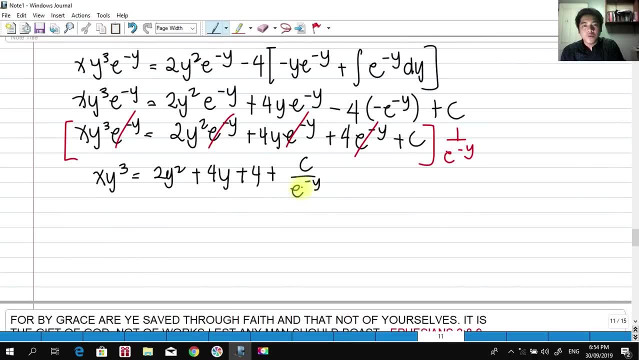 Plus 4y, Plus 4.. Plus c Over e raised to negative y, And Furthermore- If I'm going To Bring this up, We will be having A positive exponent Here Of 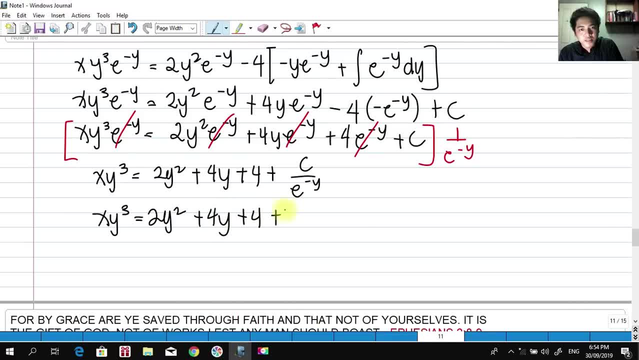 e, y, 4y Plus 4. Plus c. Okay, This Can Be The Final Answer For Our Linear Te. So Down To Our Last Example. 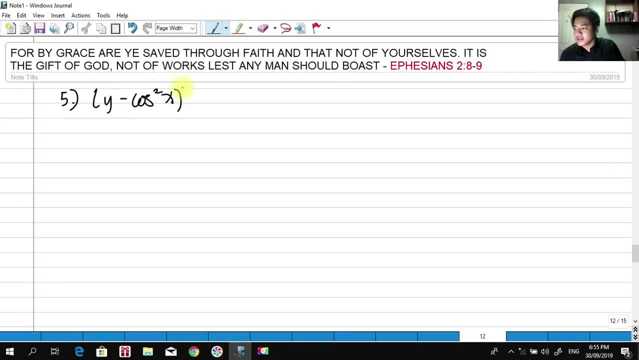 For This Video Of Linear Te, First Order, Linear Differential Equation. We Have Y D X Minus Cosine Squared X D X Plus Cosine. 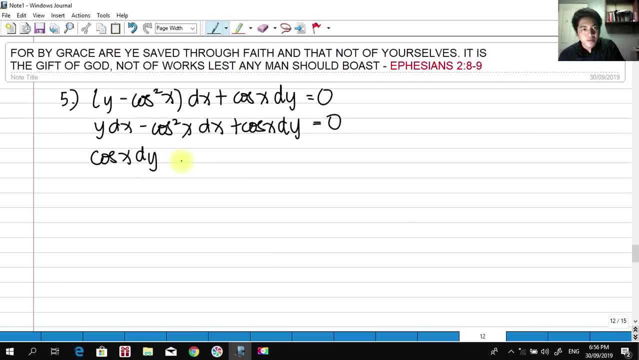 Of X, D, Y Plus Y D, X Minus Cosine Of Squared X- D, X Is Equals To Multiply The Equation By One Over. 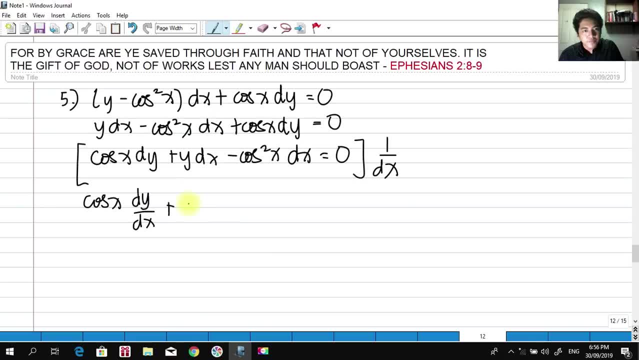 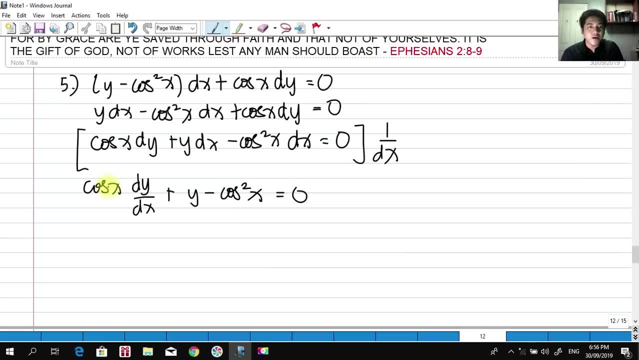 D X. I'm Going To Eliminate D X. Here We Have Cosine Of X, D Y Over D X Plus Y Minus The D. 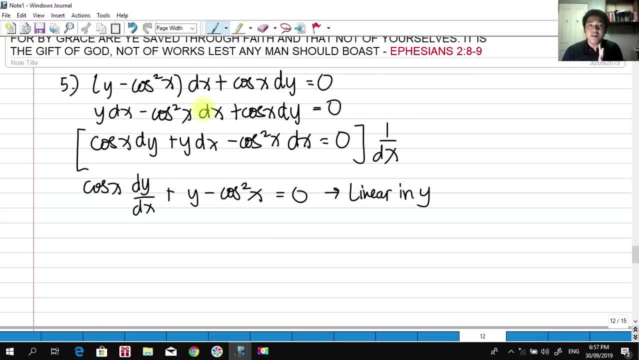 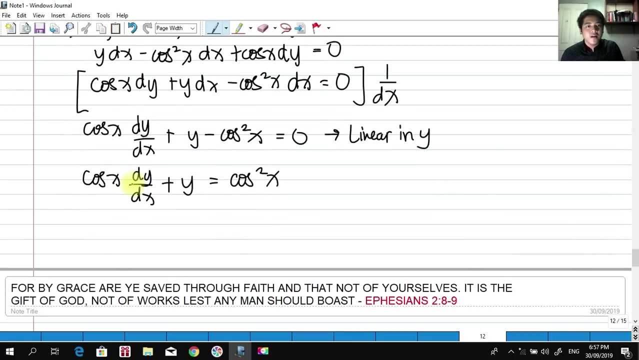 X Here We Have Two Terms Of D X Here, Then Definitely That Is Not Linear In X, Whereas We Only Have One Term Of D. 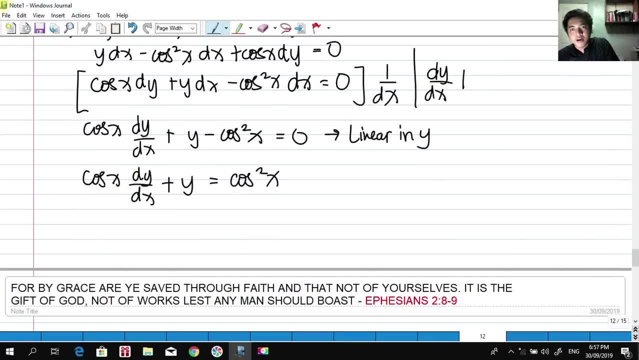 Y Is D Y Over D X, Plus Again P Of X Times Y Is Equals To Q Of X. Okay, And I'm Going To. 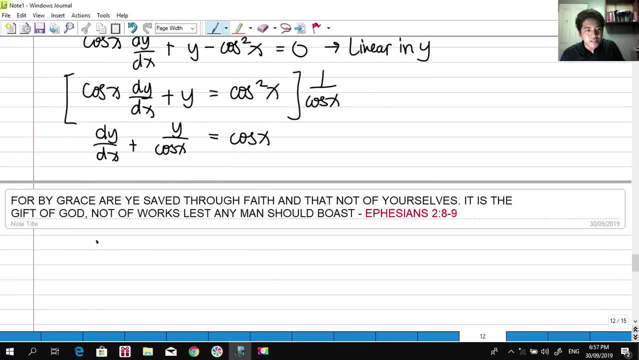 Divide This By One Over D X Plus One Over Cosine Of X, Multiplied By Y Is Equals To Cosine Of X, As You. 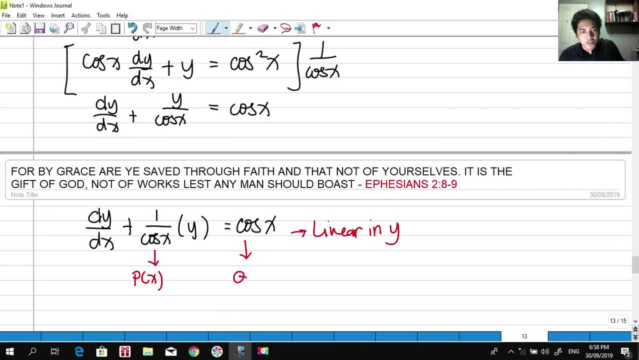 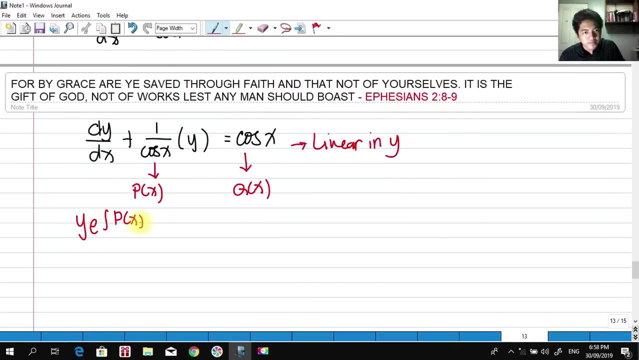 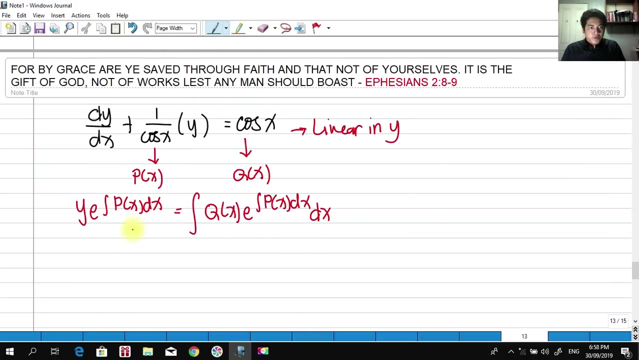 Can See. This Is The Linear In Linear In Y Of X, D. X Is Equal To The Integral Of Q Of X Multiplied By. 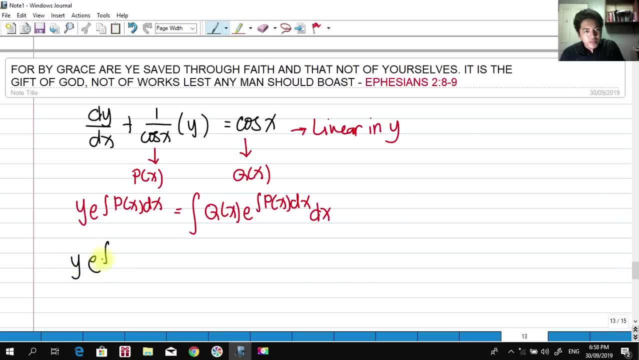 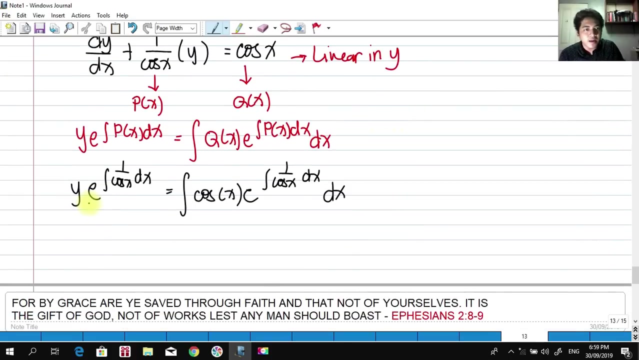 E Is To Integral Of P, Of X, D, X And We Have The X Multiplied By E Is The Integral Of One Over Cosine. 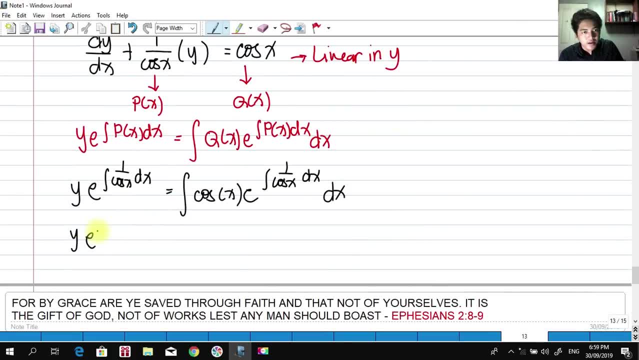 Of X D X And We Have The X Here And One Over Cosine Of X Is Equal To The Integral Of X D X. 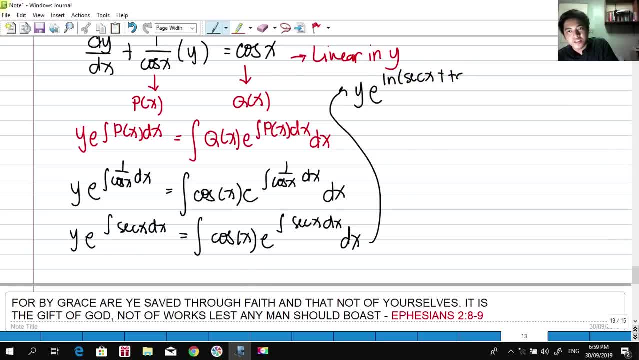 Is L? N Second Of X, Plus Tangent Of X Is Equal To Integral Of Cosine Of X. Okay, E Is To L N Will. 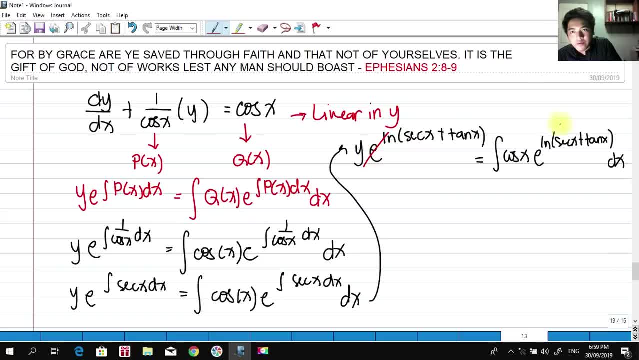 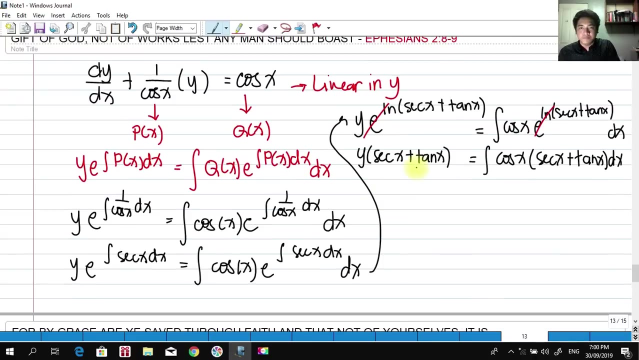 Cancel Here. So What Will Happen To The Equation? We Have Y Second Of X Plus Tangent Of X. Here Is Equal. Now To The 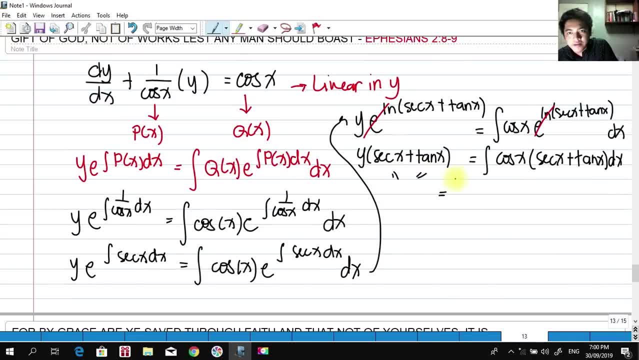 Integral Of Cosine Of X. This Should Be Cosine Of X Multiplied By Second Of X, Plus The Integral Of Cosine Of X Multiplied. 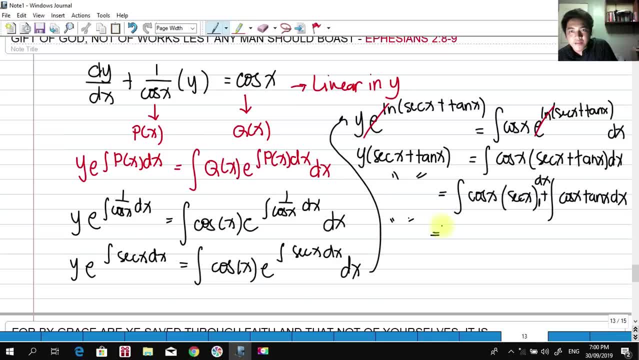 By Tangent Of X, D, X. So Definitely This Would Cancel Plus Cosine Of X Tangent Is Equal To Sine Of X Over Cosine.